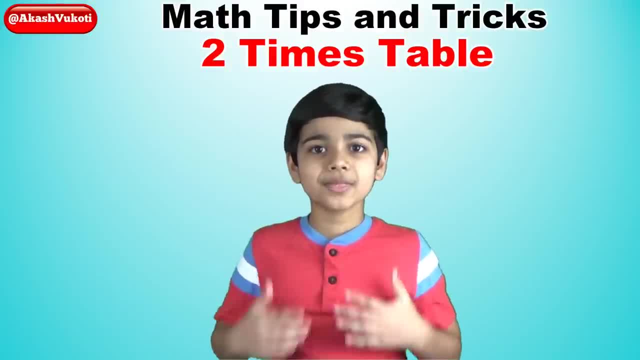 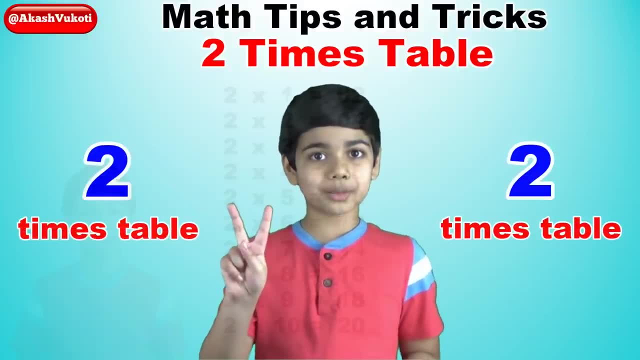 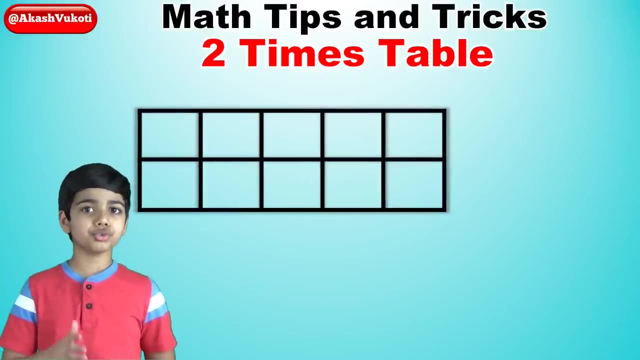 Hello friends, I'm Akash. Today in the Math Tips and Tricks series, we're going to be learning the trick for the 2x table. Let's begin by drawing out a 5x2 grid of 5 columns and 2 rows. 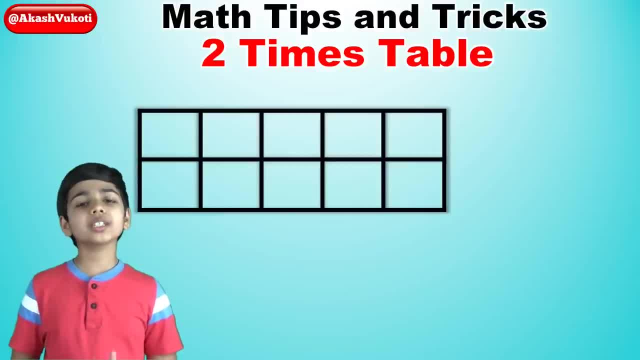 Next, for the ones digits, write the 2x table, from 2x1,, which is 2,, to 2x4,, which is 8.. Then we write a 0. You may remember 2 to 8 from, well, the 2x table that I just mentioned. 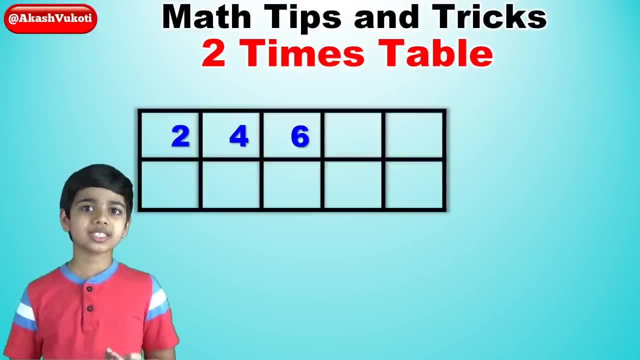 So 2,, 4,, 6,, 8,, 0.. Remember to add a 0 at the end, And then do the same for the bottom row too. So 2,, 4,, 6,, 8, 0.. 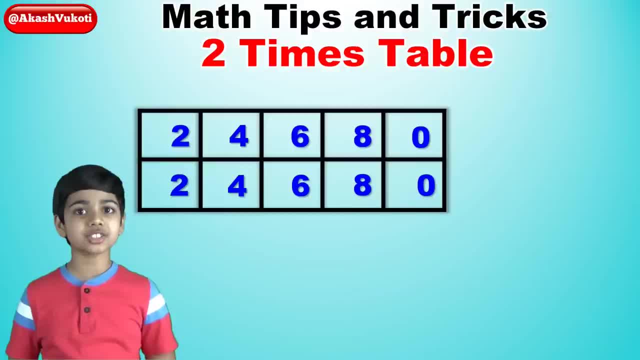 So now we can split the tens digits into two parts, Top row and bottom row. For the tens digits in the top row, we will write 0 in all boxes except the last one. We will write 1 in that box. So 0, 0, 0, 0, 1.. 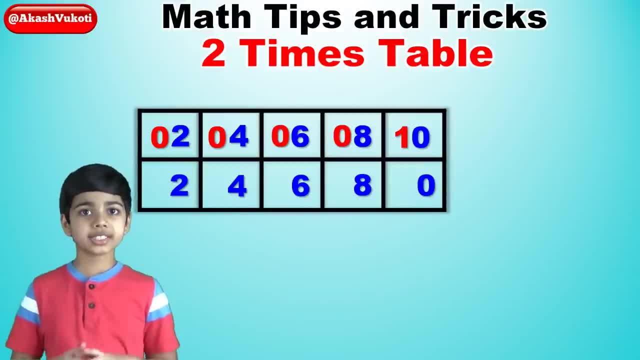 And now for the tens digits in the bottom row. similar setup: we write 1 in all boxes except the last one. We will write 2 in the last box instead of 1.. So 1, 1, 1, 1, 2.. 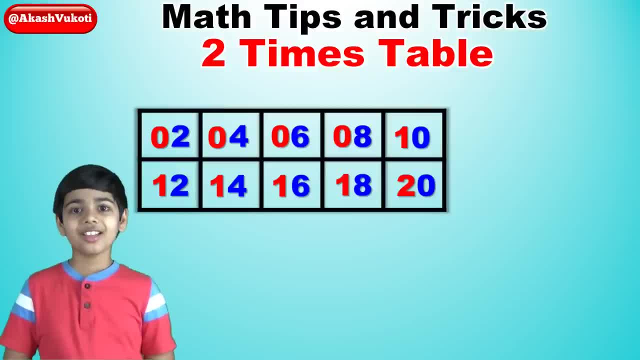 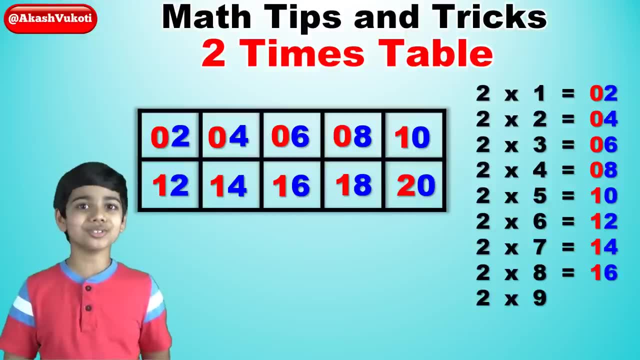 And now you have. this is amazing. you have the 2x table. Check this out. It's a really neat way to learn the 2x table, And that's about it. Now you have learned the trick to memorizing the 2x table. 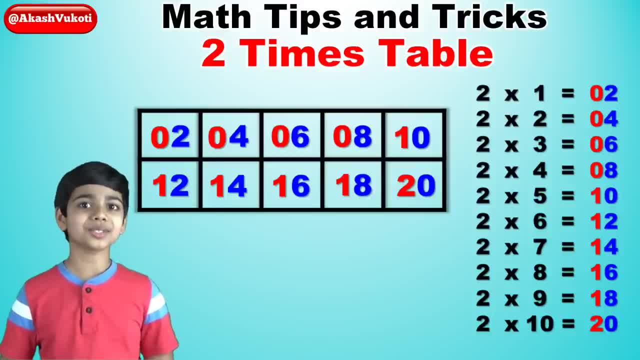 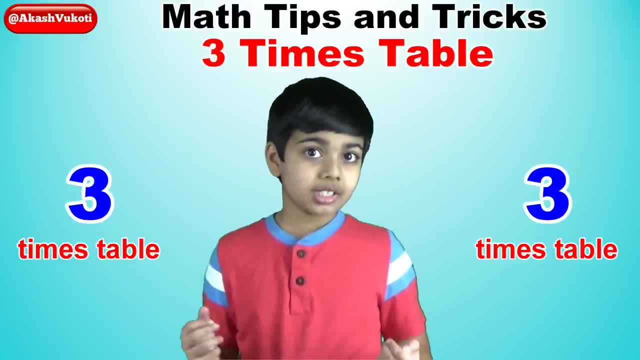 You can use it to master the 2x table. Today we are going to learn the math trick for the 3x table. The reason why I'm doing 3, because if you know this trick for the 3x table, 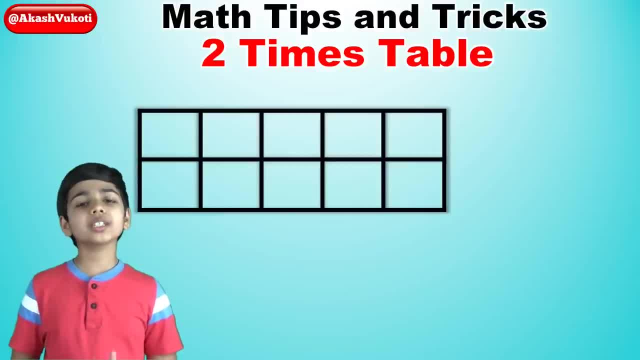 Next, for the ones digits, write the 2x table, from 2x1,, which is 2,, to 2x4,, which is 8.. Then we write a 0. You may remember 2 to 8 from, well, the 2x table that I just mentioned. 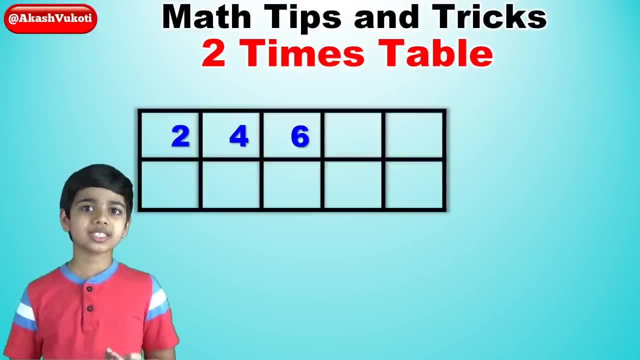 So 2,, 4,, 6,, 8,, 0.. Remember to add a 0 at the end, And then do the same for the bottom row too. So 2,, 4,, 6,, 8, 0.. 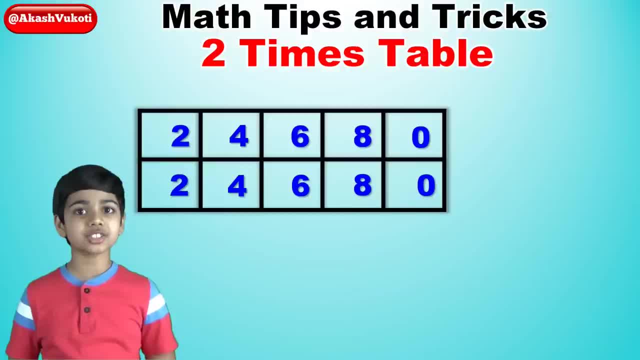 So now we can split the tens digits into two parts, Top row and bottom row. For the tens digits in the top row, we will write 0 in all boxes except the last one. We will write 1 in that box. So 0, 0, 0, 0, 1.. 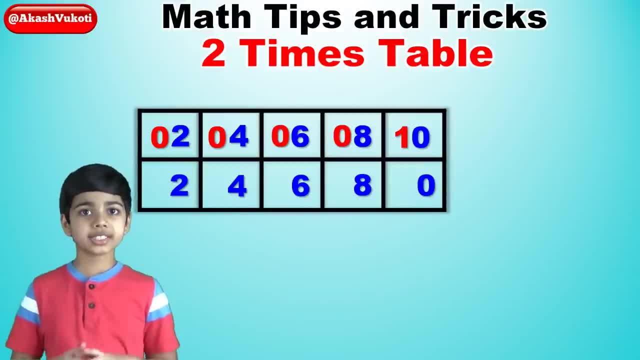 And now for the tens digits in the bottom row. similar setup: we write 1 in all boxes except the last one. We will write 2 in the last box instead of 1.. So 1, 1, 1, 1, 2.. 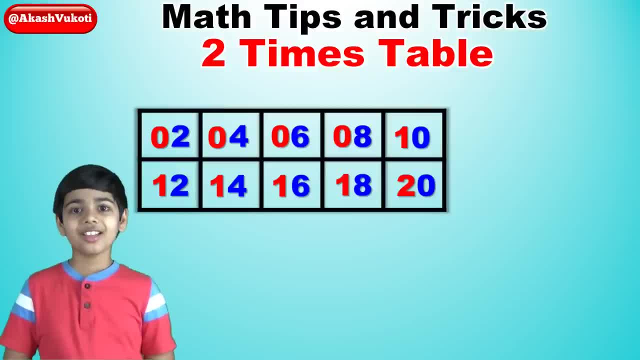 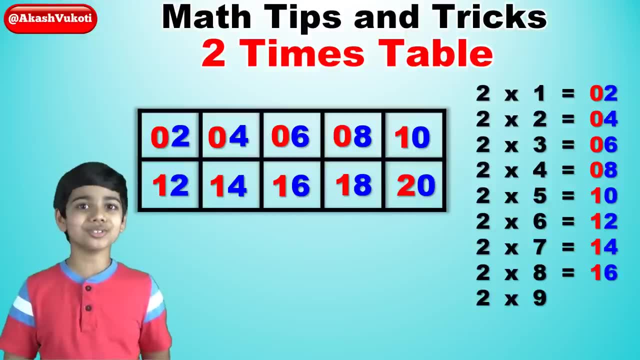 And now you have. this is amazing. you have the 2x table. Check this out. It's a really neat way to learn the 2x table, And that's about it. Now you have learned the trick to memorizing the 2x table. 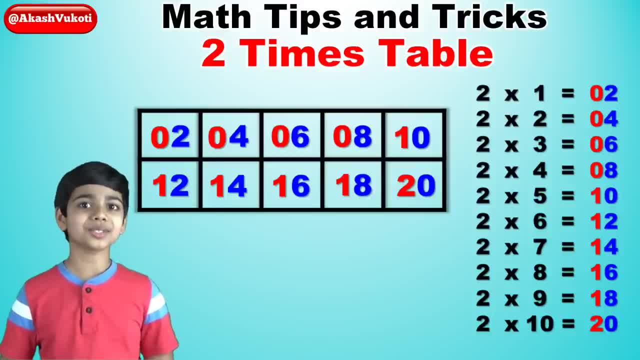 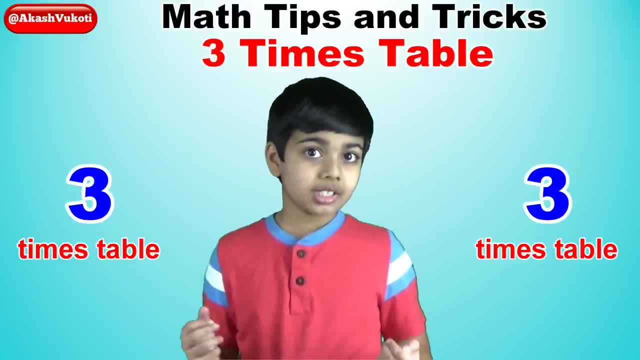 You can use it to master the 2x table. Today we are going to learn the math trick for the 3x table. The reason why I'm doing 3, because if you know this trick for the 3x table, 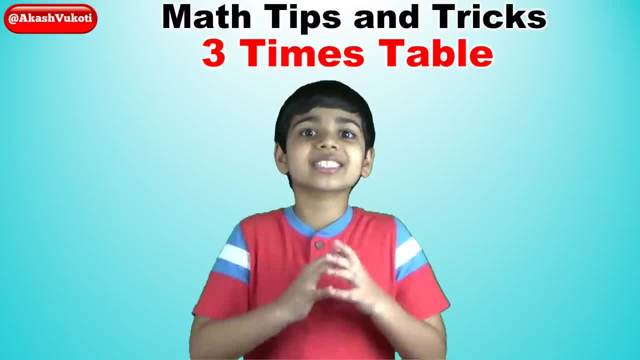 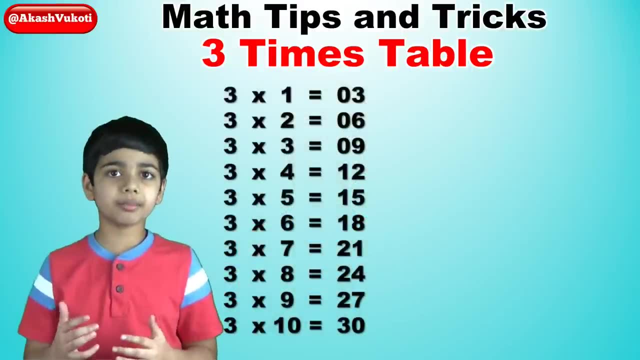 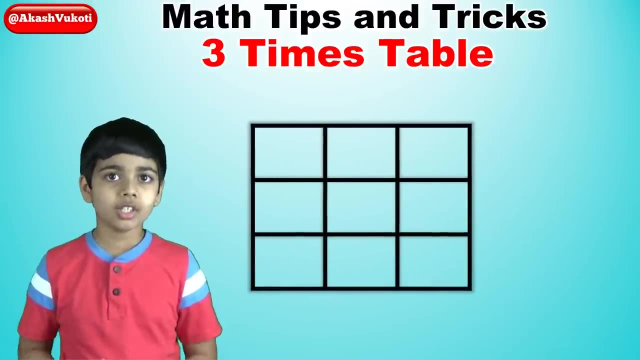 you will easily be able to learn the 6x table using a variation of this trick. I'll explain that later. Let's begin by drawing out a 3x3 tic-tac-toe grid. Now we can start For the ones digits. we go to the bottom left box and write down the numbers from 1 to 9. 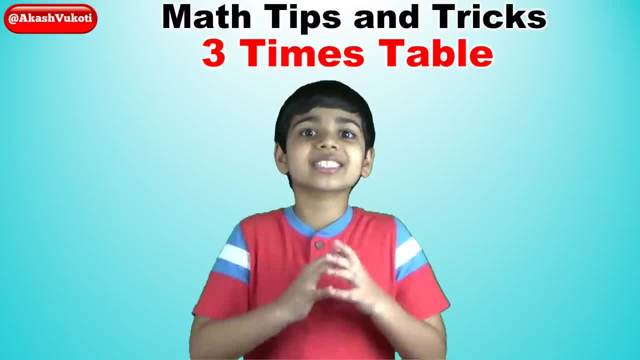 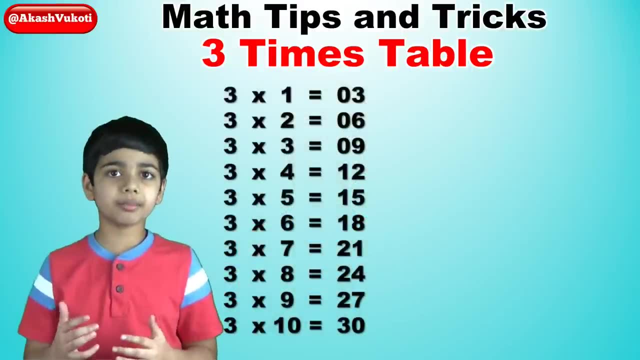 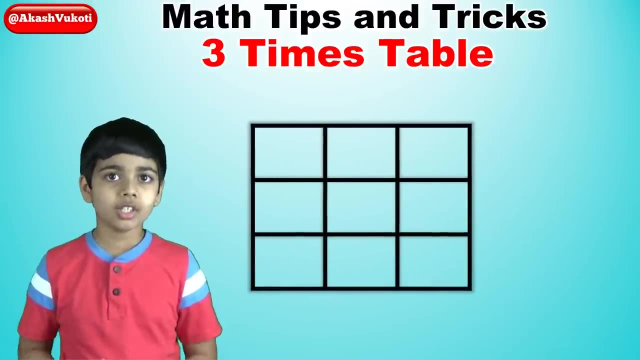 you will easily be able to learn the 6x table using a variation of this trick. I'll explain that later. Let's begin by drawing out a 3x3 tic-tac-toe grid. Now we can start For the ones digits. we go to the bottom left box and write down the numbers from 1 to 9. 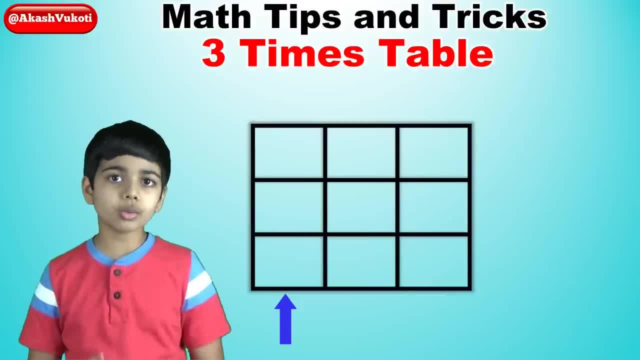 by starting in the leftmost column and going forward to the rightmost column, But this time we're going to go up from the bottom box to the top of the column. So 1,, 2,, 3,, 4,, 5,, 6,, 7,, 8,, 9,, 10.. 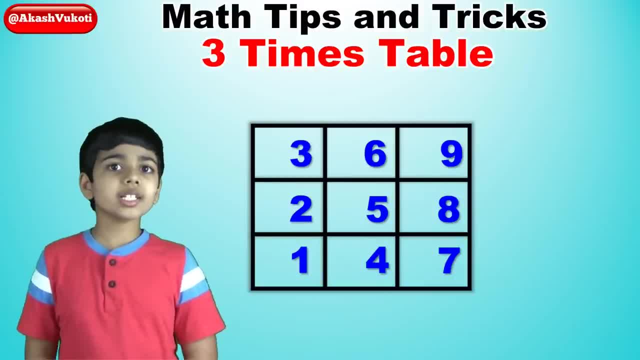 And then write a 0 to the right of the bottom row. Now for the tens digits. we're going to split this up into three sections: Top row, middle row, bottom row. For the tens digits. in the top row we write 0.. 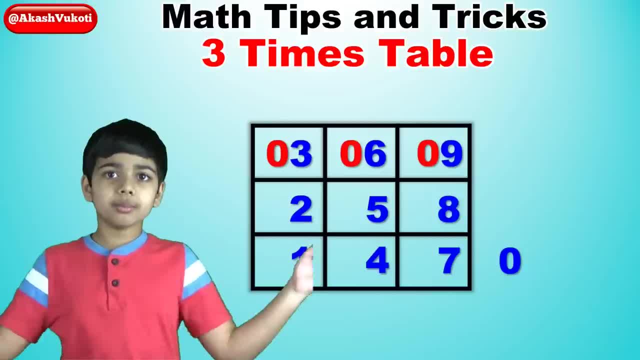 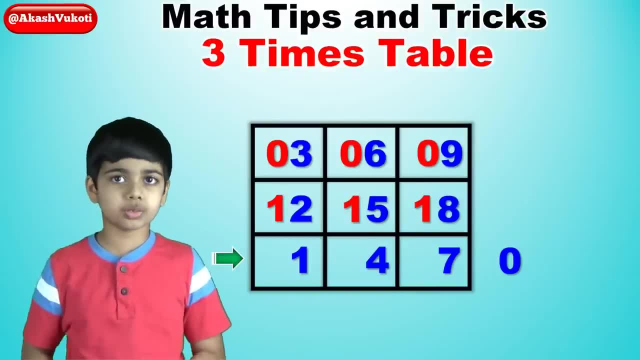 So 0, 0, 0.. For the tens digits in the middle row, we write 1.. So 1, 1, 1.. And then, for the bottom row tens digits, we're going to write 2.. 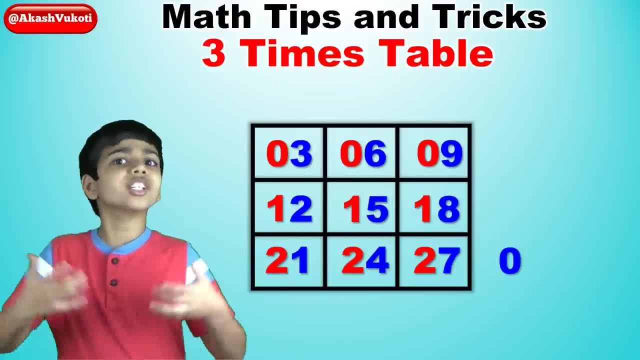 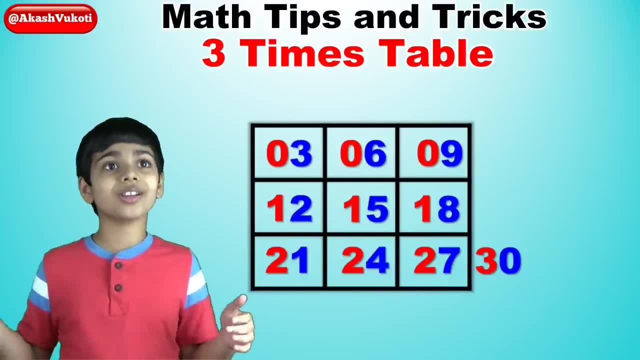 2,, 2,, 2.. And then we write a 3 next to the 0 to get 30, which you may know is 3x10.. And now you have the 3x table. Take a look, This is a really awesome trick, I'd say. 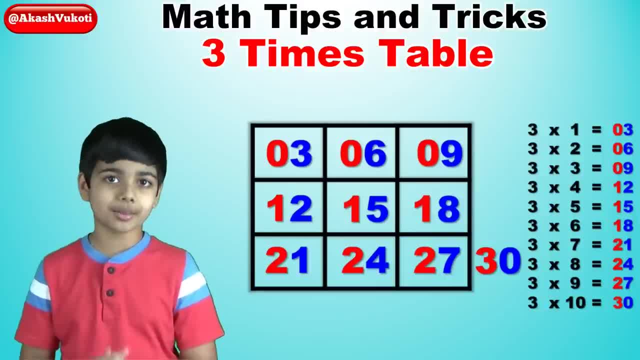 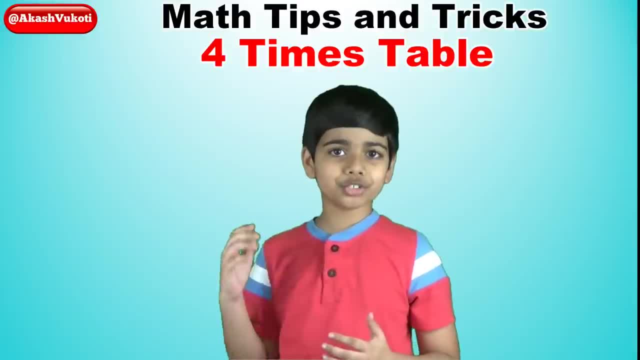 So now you know the trick to learn the 3x table, You can use it to start memorizing the 3x table. In the Math Tips and Tricks section in the Math Tips and Tricks series, we're going to learn the trick for the 4x table. 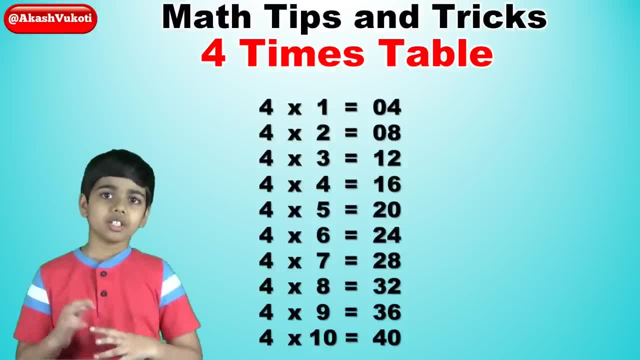 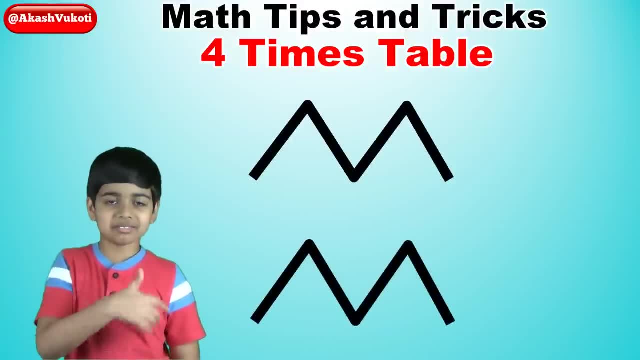 So now we can actually start Draw out two upside-down W's, or rather just draw out two M's kind of Like here, as you can see behind me, Then write the 2x table from 2 to 8,. 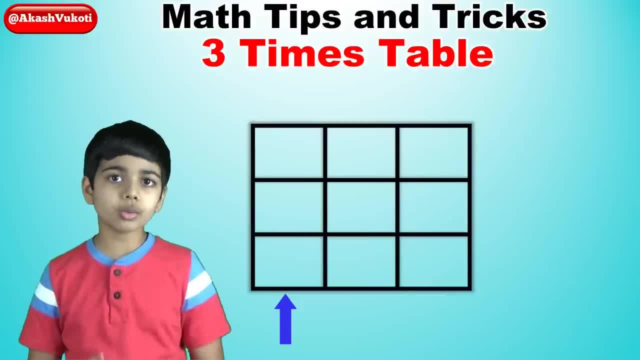 by starting in the leftmost column and going forward to the rightmost column, But this time we're going to go up from the bottom box to the top of the column. So 1,, 2,, 3,, 4,, 5,, 6,, 7,, 8,, 9,, 10.. 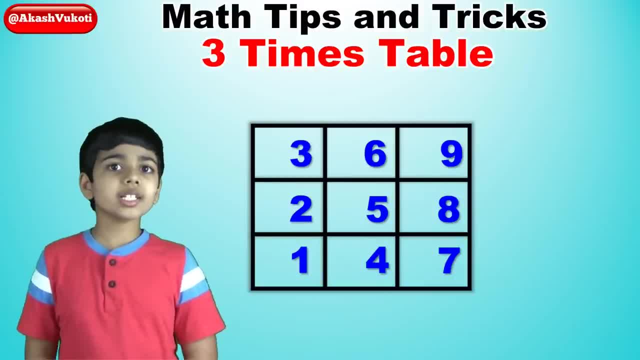 And then write a 0 to the right of the bottom row. Now for the tens digits. we're going to split this up into three sections: Top row, middle row, bottom row. For the tens digits. in the top row we write 0.. 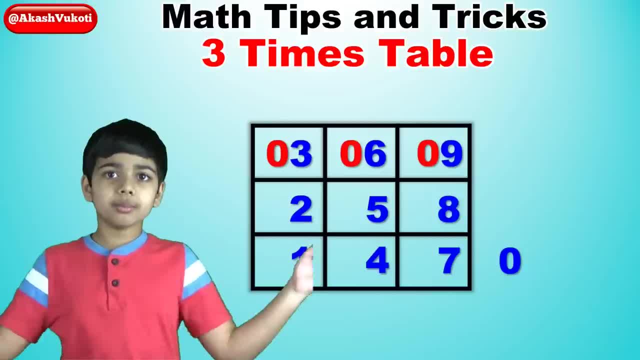 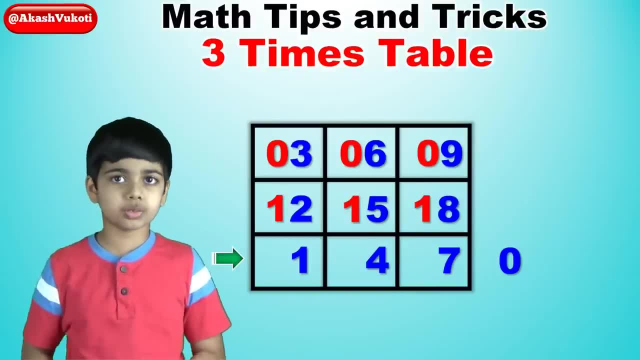 So 0, 0, 0.. For the tens digits in the middle row, we write 1.. So 1, 1, 1.. And then, for the bottom row tens digits, we're going to write 2.. 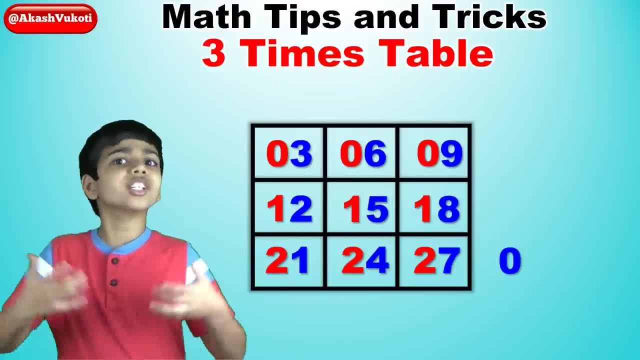 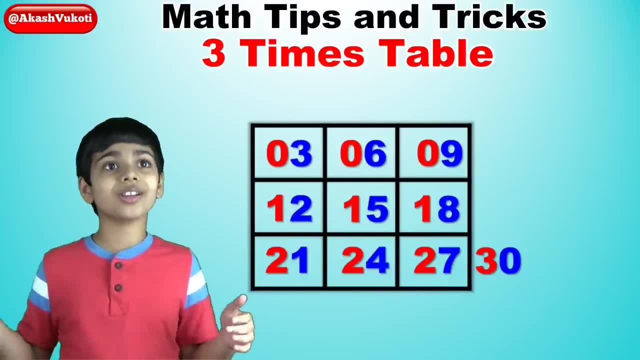 2,, 2,, 2.. And then we write a 3 next to the 0 to get 30, which you may know is 3x10.. And now you have the 3x table. Take a look, This is a really awesome trick, I'd say. 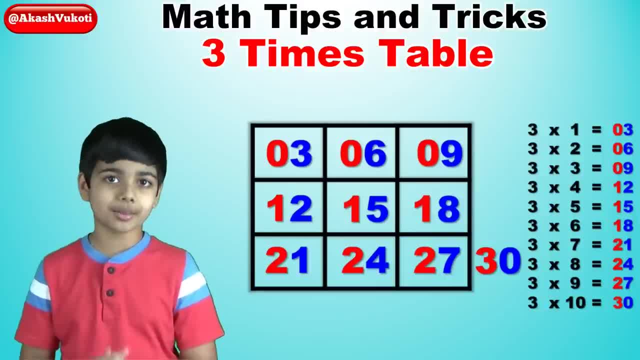 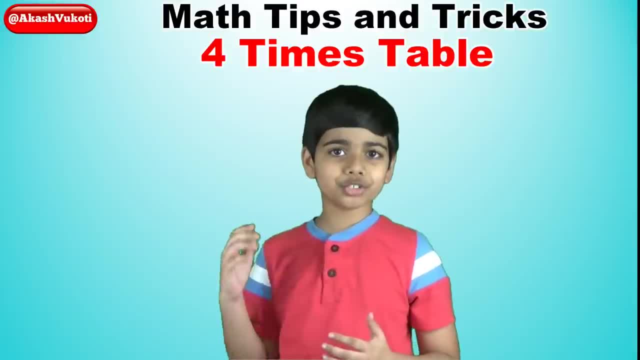 So now you know the trick to learn the 3x table, You can use it to start memorizing the 3x table. In the Math Tips and Tricks section in the Math Tips and Tricks series, we're going to learn the trick for the 4x table. 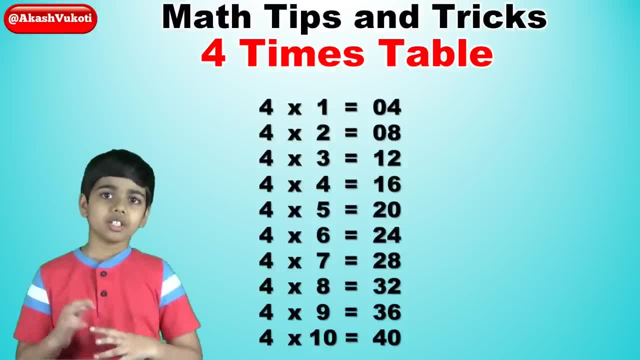 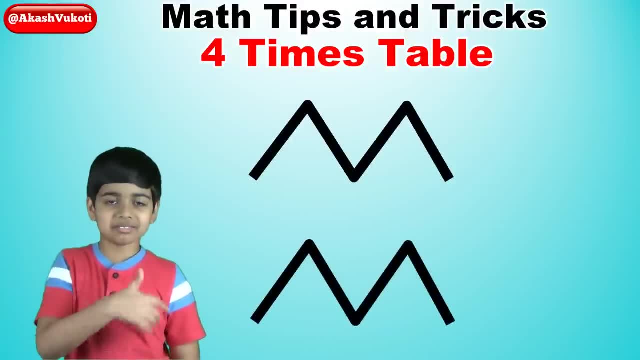 So now we can actually start Draw out two upside-down W's, or rather just draw out two M's kind of Like here, as you can see behind me, Then write the 2x table from 2 to 8,. 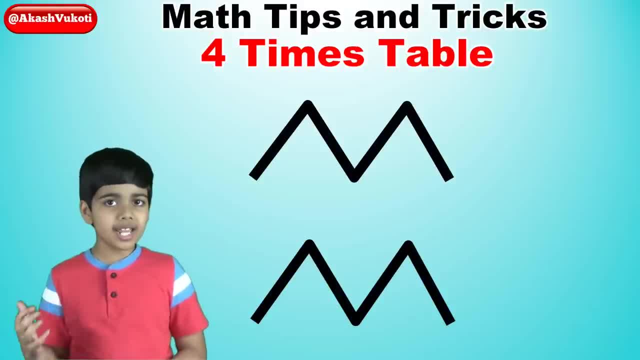 followed by a 0 at each point of the M. So this follows the pattern 2, 4, 6, 8, 0. So 2, 4, 6, 8, 0. And then the same for the other one. 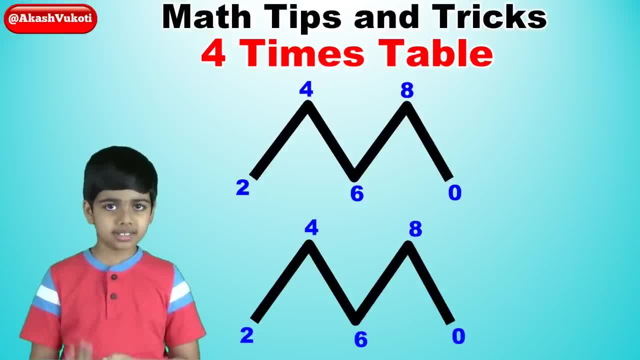 2,, 4,, 6,, 8,, 0.. Now that's the ones digits done. Now we can split the tens digits into four sections: The top row of the first M. the bottom row of the first M. 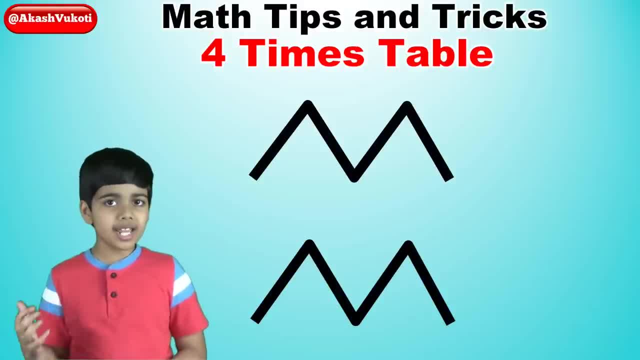 followed by a 0 at each point of the M. So this follows the pattern 2, 4, 6, 8, 0. So 2, 4, 6, 8, 0. And then the same for the other one. 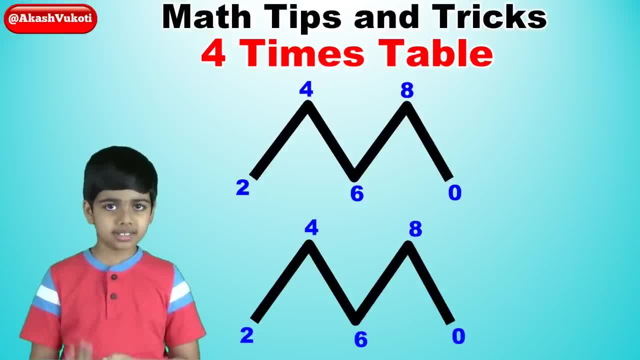 2,, 4,, 6,, 8,, 0.. Now that's the ones digits done. Now we can split the tens digits into four sections: The top row of the first M. the bottom row of the first M. 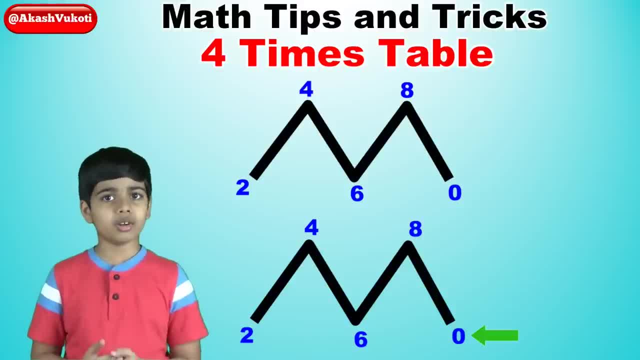 the top row of the second M and the bottom row of the second M. For the top row of the first M, just write 0.. So 0, 0.. For the bottom row of the first M, write 1, except for the last one. 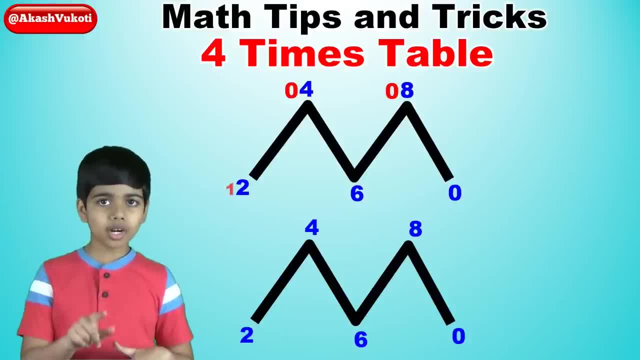 There we write 2.. So 1, 1, 2.. For the top row of the second M, just write 2.. So 2, 2.. And for the bottom row of the second M write 3, except for the last one. 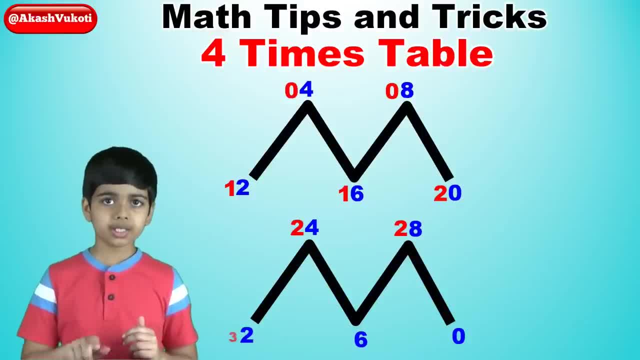 There we write 4.. So 3,, 3,, 4.. And so, right before your very eyes, you have completed the 4x table. This is a very neat trick, to memorize it and, as you can see, 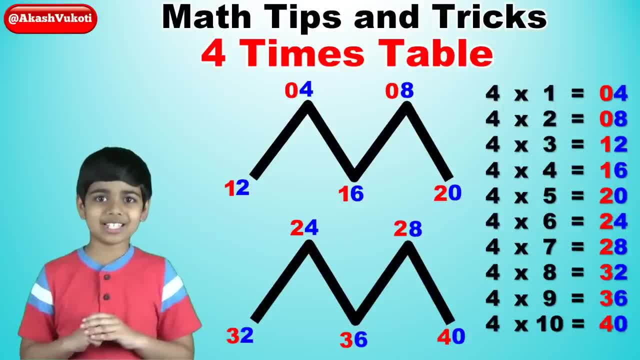 right here behind me, just look at it. It's really, really neat And it's a really good way to learn the 4x table. And that's about it. Now you have learned the trick to memorize the 4x table. 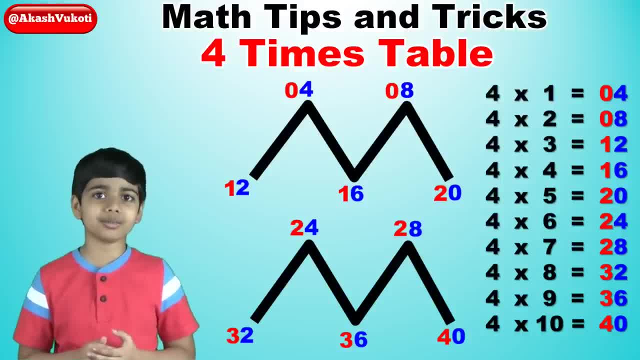 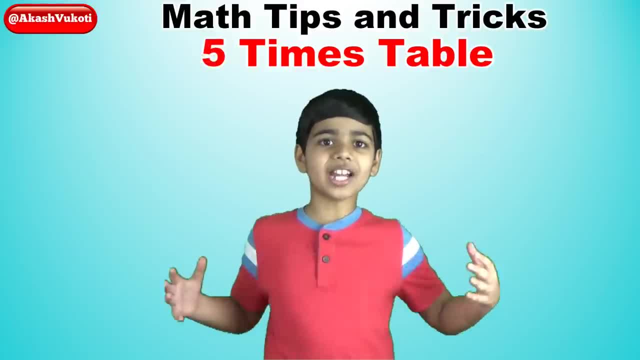 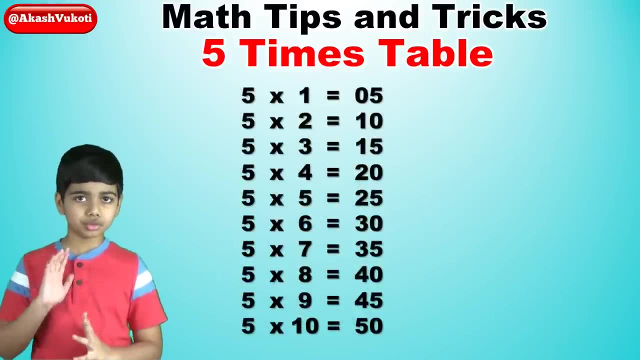 You can use it to master the 4x table. Today in the Math Tips and Tricks series, we're going to learn the trick for the 5x table. Now we can start. Draw out a 5x2 grid of 5 columns and 2 rows. 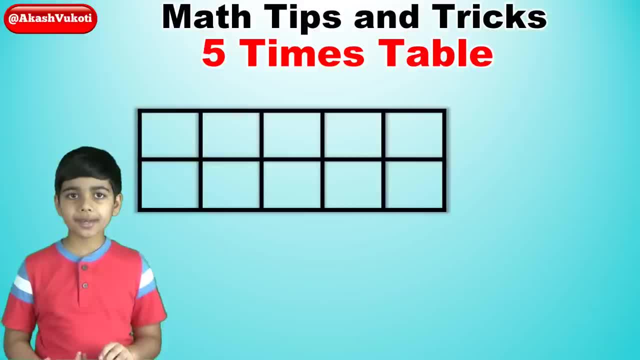 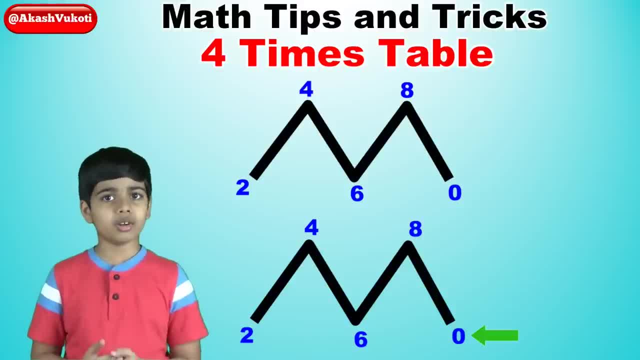 the top row of the second M and the bottom row of the second M. For the top row of the first M, just write 0.. So 0, 0.. For the bottom row of the first M, write 1, except for the last one. 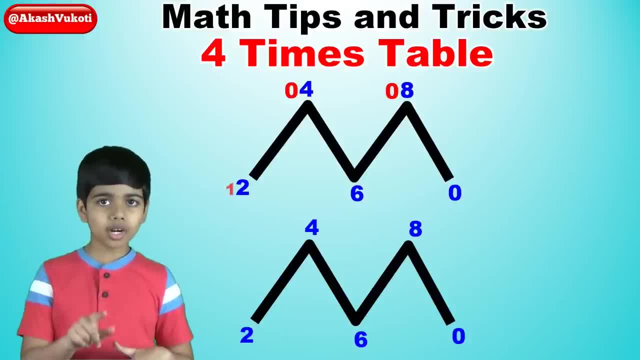 There we write 2.. So 1, 1, 2.. For the top row of the second M, just write 2.. So 2, 2.. And for the bottom row of the second M write 3, except for the last one. 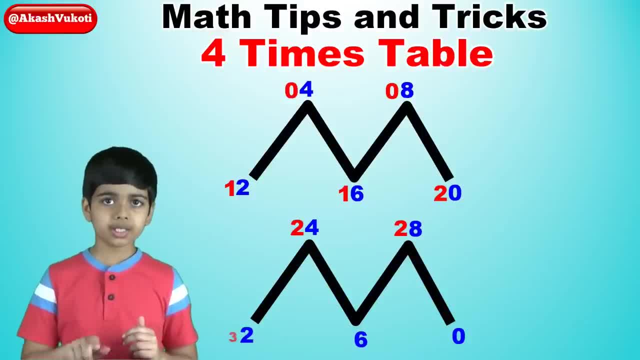 There we write 4.. So 3,, 3,, 4.. And so, right before your very eyes, you have completed the 4x table. This is a very neat trick, to memorize it and, as you can see, 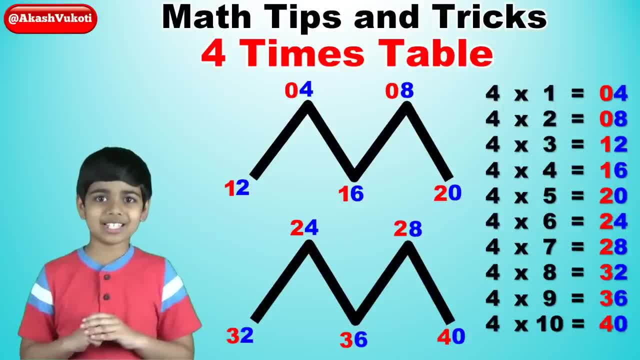 right here behind me, just look at it. It's really, really neat And it's a really good way to learn the 4x table. And that's about it. Now you have learned the trick to memorize the 4x table. 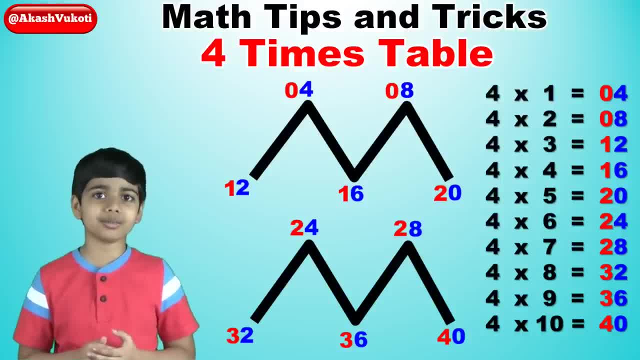 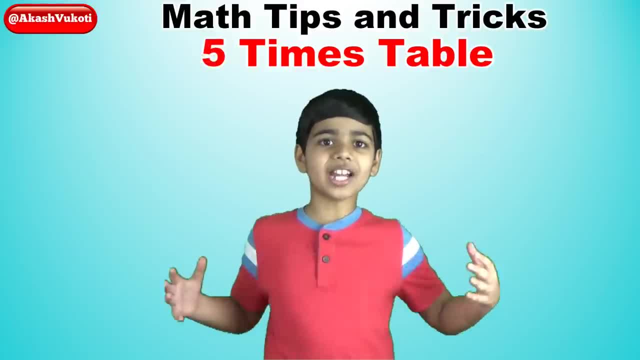 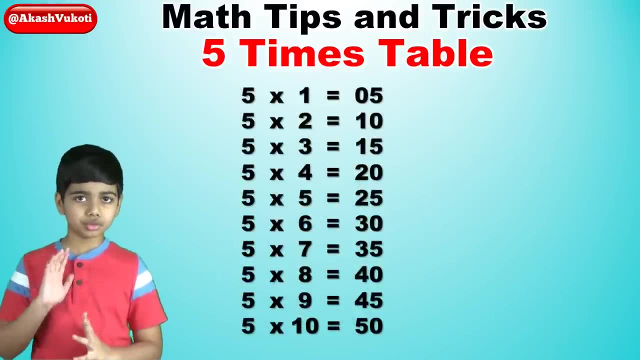 You can use it to master the 4x table. Today in the Math Tips and Tricks series, we're going to learn the trick for the 5x table. Now we can start. Draw out a 5x2 grid of 5 columns and 2 rows. 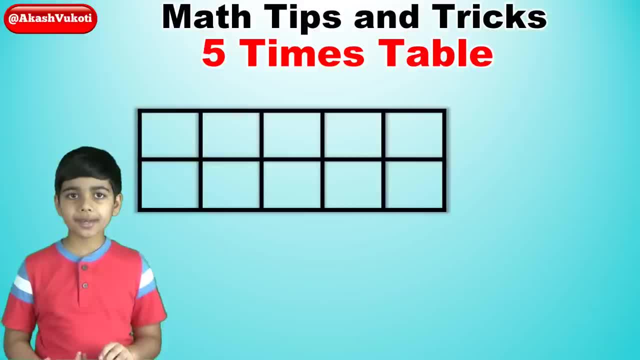 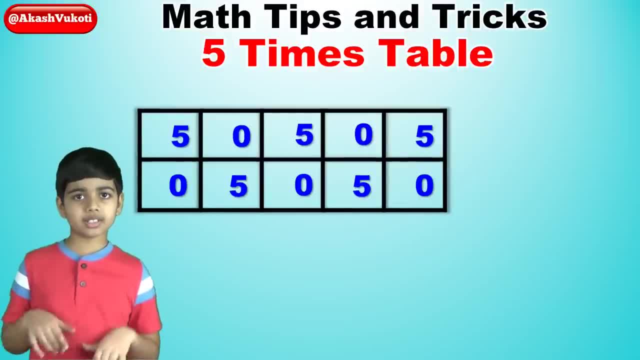 For the tens digits, you write a 0,, and then each number from 1 to 4, twice, And then, finally, you write the number 5 in the boxes. So this is the pattern: 0, 1,, 1,, 2,, 2,, 3,, 3, 4,, 4, 5.. 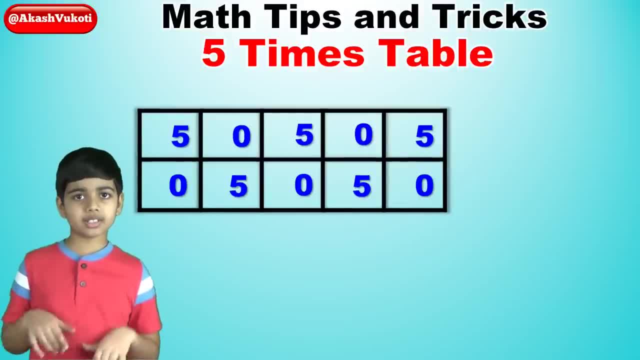 For the tens digits, you write a 0,, and then each number from 1 to 4, twice, And then, finally, you write the number 5 in the boxes. So this is the pattern: 0, 1,, 1,, 2,, 2,, 3,, 3, 4,, 4, 5.. 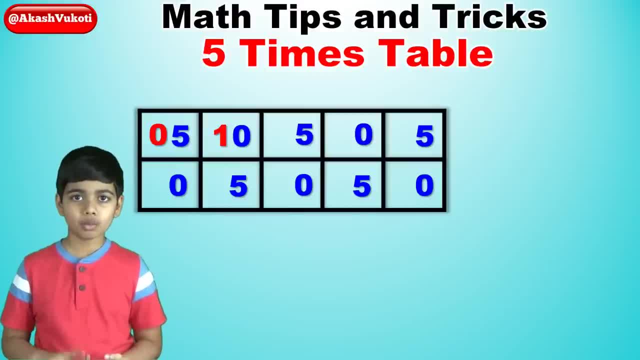 And so let's do that: 0, 1,, 1,, 2,, 2,, 3,, 3,, 4,, 4,, 5.. And now you have the 5x table. Check this out. 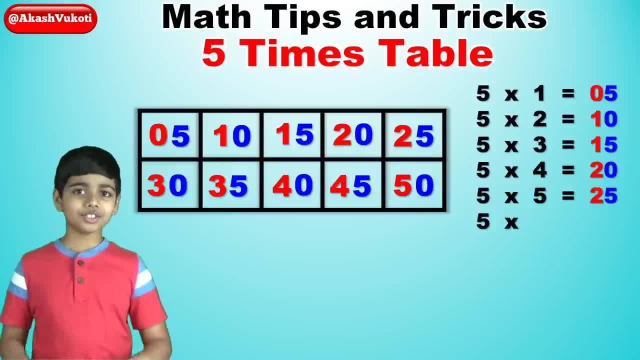 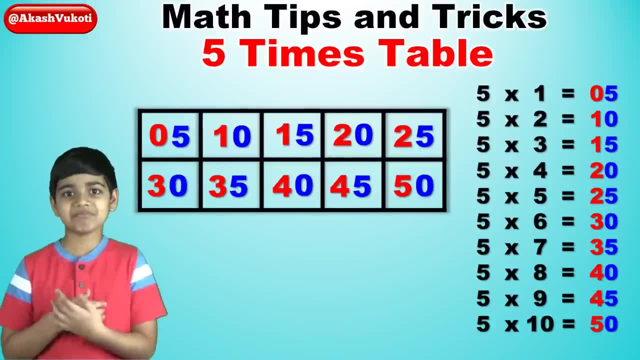 This is a really neat way to learn the 5x table, And you can see it goes from 5x1 to 5x10.. That is the 5x table, And that's about it. Now you have learned the trick. 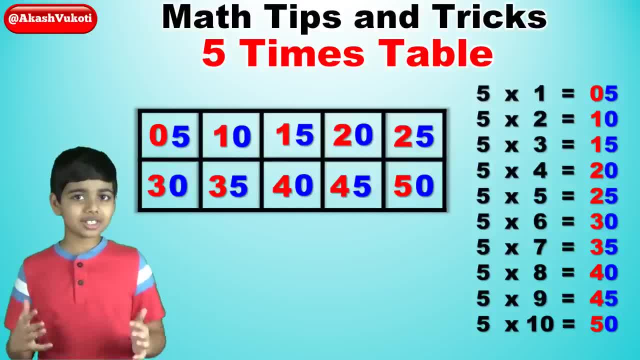 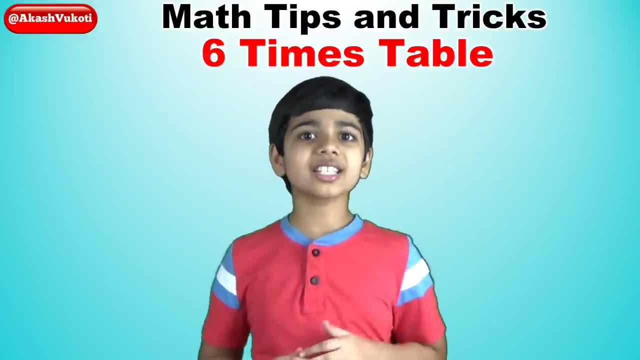 to memorize the 5x table. You can use it to master the 5x table. In the 3x table trick video I said that if you learned the 3x table trick, you would easily learn the 6x table trick. 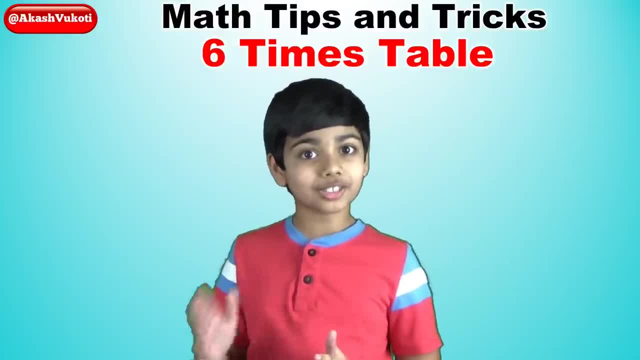 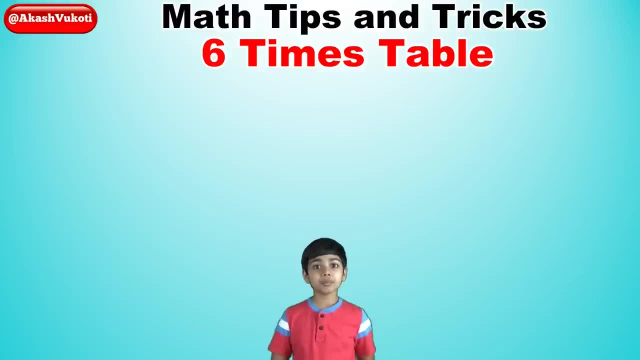 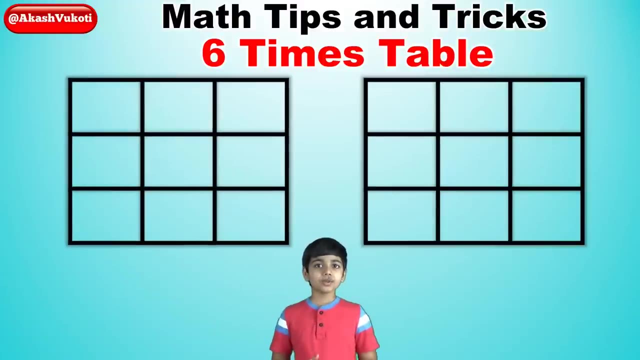 With one that's just much like it. So today we're going to show you that 6x table trick. Let's begin by drawing out two tic-tac-toe grids, One next to the other. Next, we'll start from the bottom left corner. 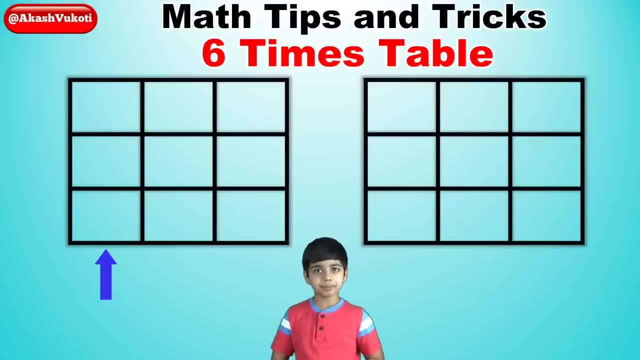 and write all the numbers from 1 to 9.. We'll start in the leftmost column, going upwards from the bottom left corner, And then we will go forwards over to the rightmost column. So 1,, 2,, 3,, 4,, 5,, 6,, 7,, 8,, 9.. 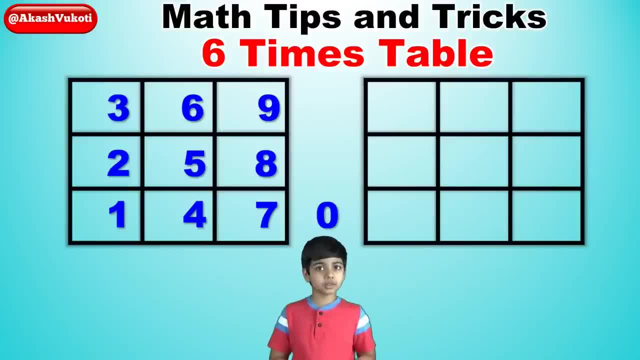 Then write a 0 next to the bottom row. So do the same for the other grid too. Now for the tens digits. we'll split the grid into three parts, each Middle row, bottom row. This is going to take a tiny bit of a while. 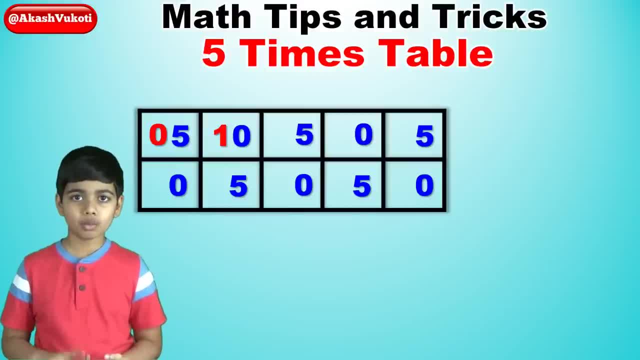 And so let's do that: 0, 1,, 1,, 2,, 2,, 3,, 3,, 4,, 4,, 5.. And now you have the 5x table. Check this out. 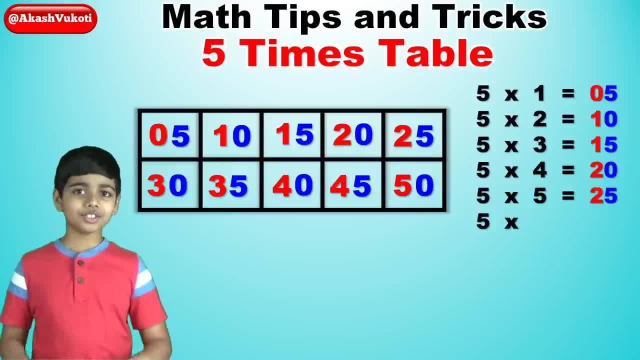 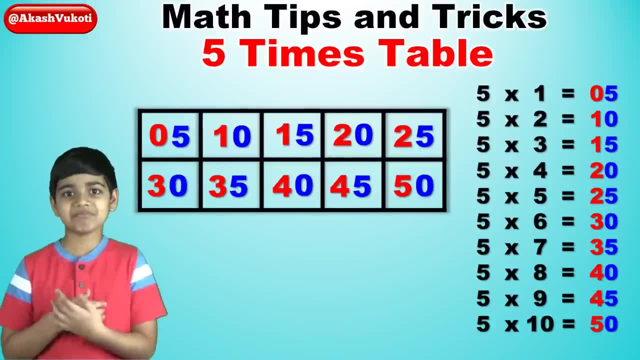 This is a really neat way to learn the 5x table, And you can see it goes from 5x1 to 5x10.. That is the 5x table, And that's about it. Now you have learned the trick. 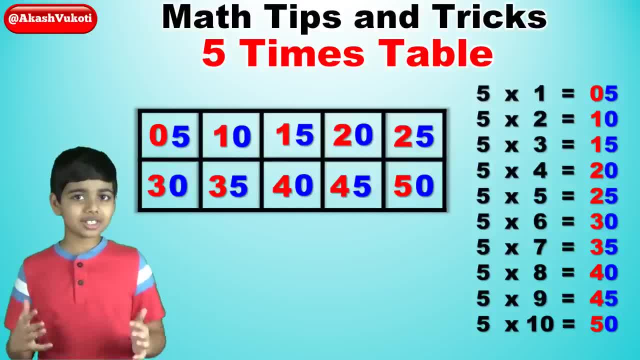 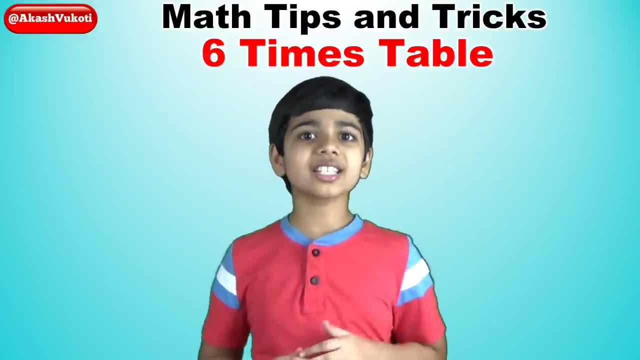 to memorize the 5x table. You can use it to master the 5x table. In the 3x table trick video I said that if you learned the 3x table trick, you would easily learn the 6x table trick. 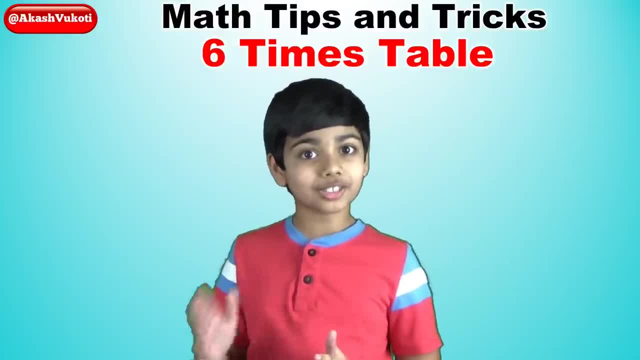 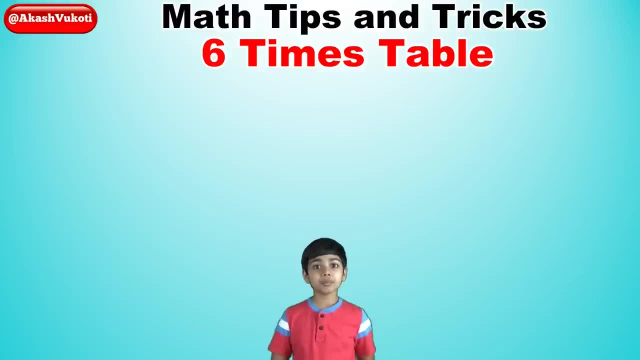 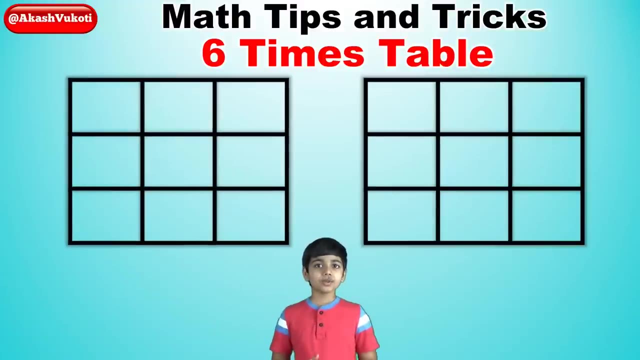 With one that's just much like it. So today we're going to show you that 6x table trick. Let's begin by drawing out two tic-tac-toe grids, One next to the other. Next, we'll start from the bottom left corner. 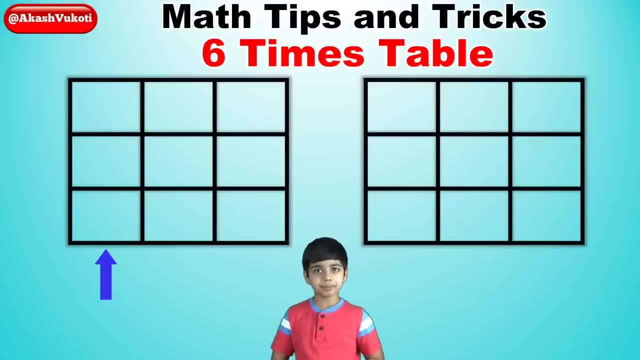 and write all the numbers from 1 to 9.. We'll start in the leftmost column, going upwards from the bottom left corner, And then we will go forwards over to the rightmost column. So 1,, 2,, 3,, 4,, 5,, 6,, 7,, 8,, 9.. 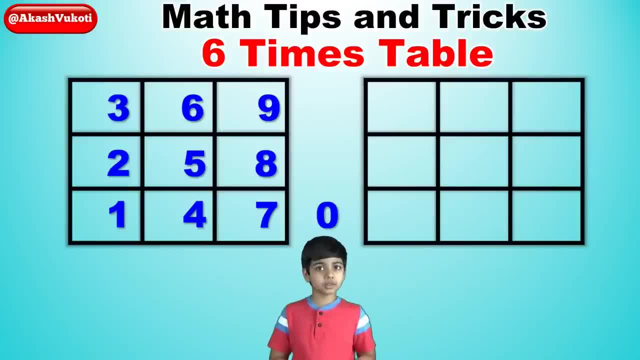 Then write a 0 next to the bottom row. So do the same for the other grid too. Now for the tens digits. we'll split the grid into three parts, each Middle row, bottom row. This is going to take a tiny bit of a while. 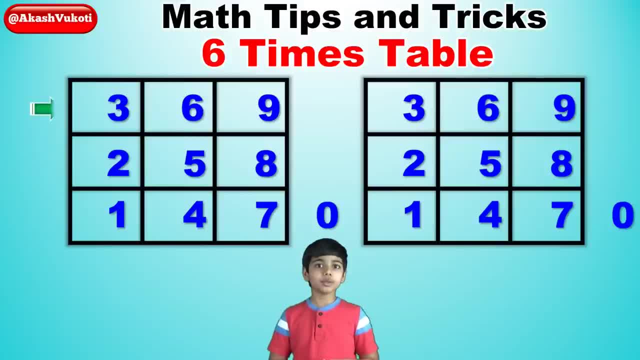 For the tens digits in the top row of the first grid, we will write 0, 0, 0.. For the tens digits in the middle row of the first grid, we will write 1, 1, 1.. For the tens digits in the bottom row: 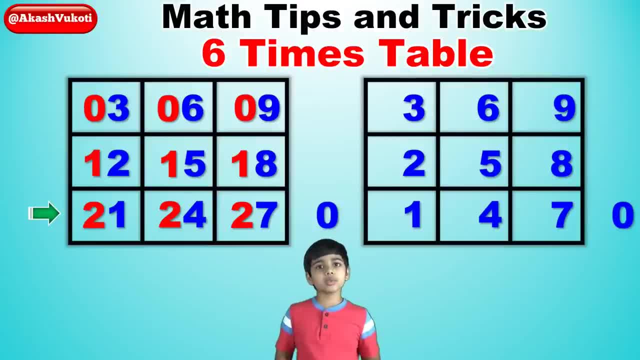 of the first grid, we write 2,, 2,, 2.. And then we write a 3 next to the first of two 0s. And then we repeat the same thing on the other side, but with different numbers this time. 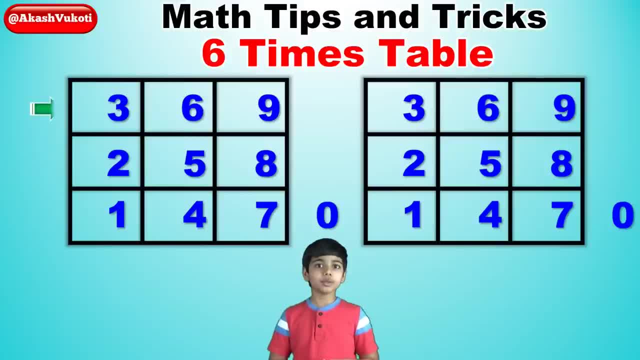 For the tens digits in the top row of the first grid, we will write 0, 0, 0.. For the tens digits in the middle row of the first grid, we will write 1, 1, 1.. For the tens digits in the bottom row: 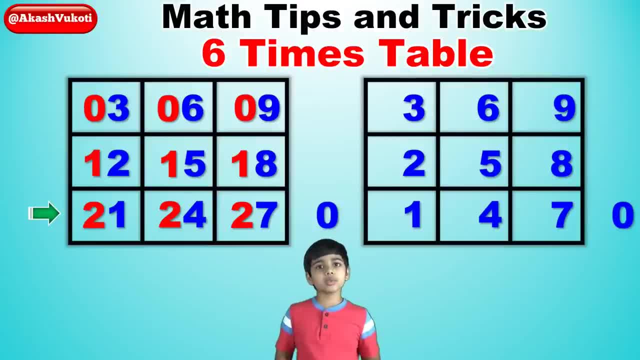 of the first grid, we write 2,, 2,, 2.. And then we write a 3 next to the first of two 0s. And then we repeat the same thing on the other side, but with different numbers this time. 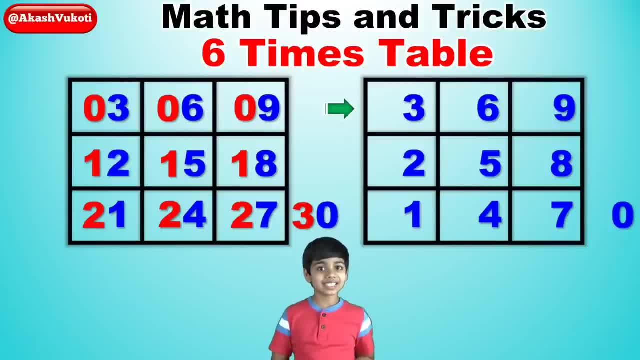 For the tens digits in the top row of the second grid, we write 3,, 3,, 3.. And I think you're going to get what's about to happen now. For the tens digits in the middle row of the second grid, we write: 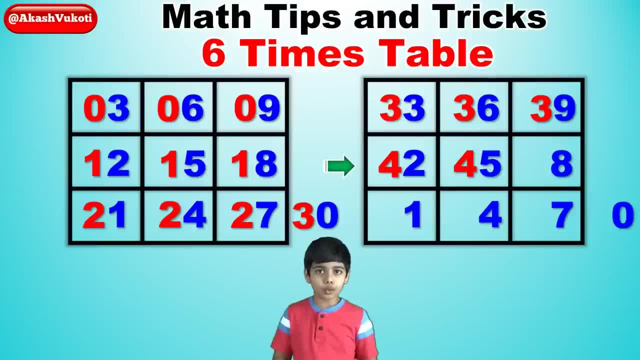 Yeah, you're pretty much right. It's 4,, 4, 4.. And for the tens digits in the bottom row of the second grid, we write 5,, 5, 5.. And then we write a 6. 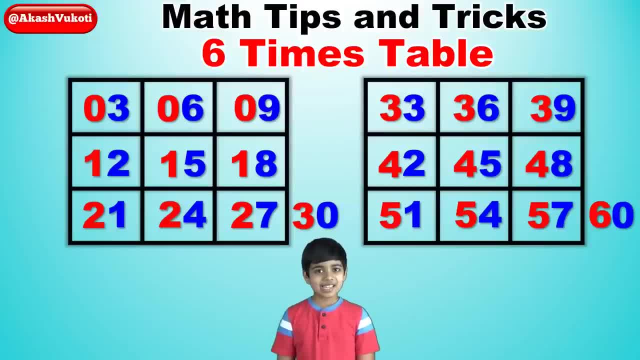 next to the second of two 0s. It sounds like a lengthy process, but you may actually notice that this is the 3 times table, from 3 times 1 to 3 times 20.. So if you know that, then well. 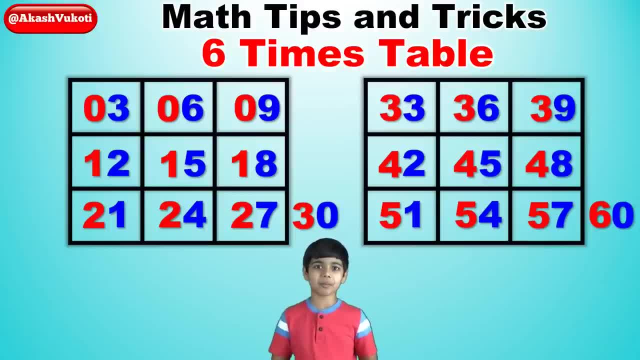 you kind of know the 6 times table using this trick. So now we can start. All you have to do is make a diamond shape in both of them and then connect the first diamond to the 30 and the second diamond to the 60.. 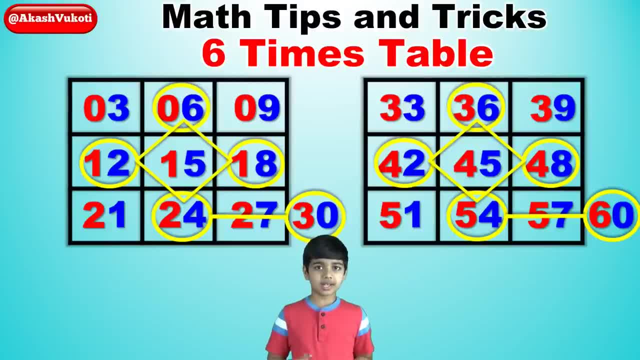 And make sure you circle all of these numbers that this diamond shape touches And all of the circled numbers create the 6 times table. Check this out. This thing is really cool. It's a really awesome trick. Yeah, this is amazing. 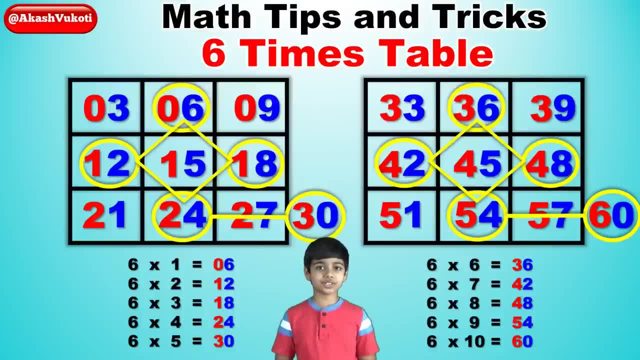 You can see behind me over there, we got the full 6 times table. It's a really awesome trick, in my opinion, really awesome. So now you know the trick to learning the 6 times table. You can use this trick. 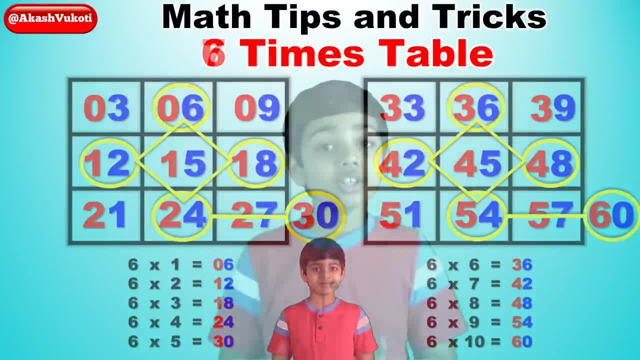 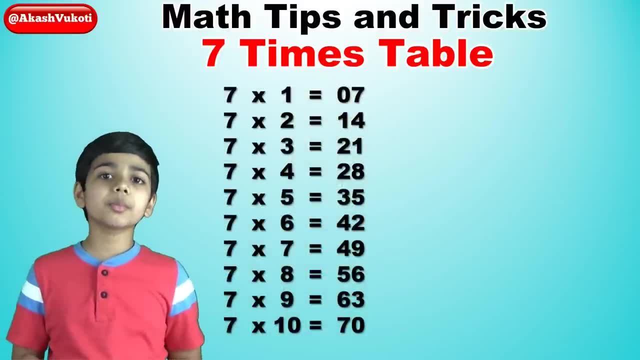 to memorize the 6 times table. We're going to learn the math trick for the 7 times table. Now let's begin by drawing out a 3 by 3 tic-tac-toe grid. as you can see behind me, 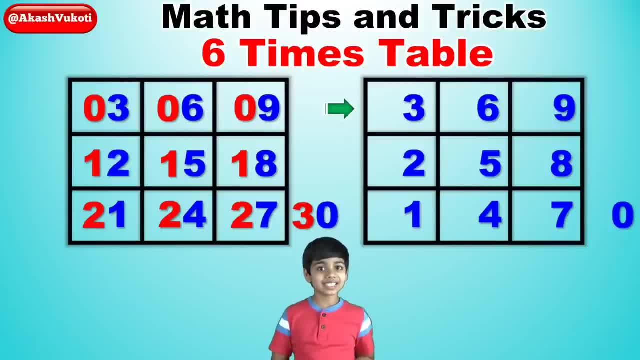 For the tens digits in the top row of the second grid, we write 3,, 3,, 3.. And I think you're going to get what's about to happen now. For the tens digits in the middle row of the second grid, we write: 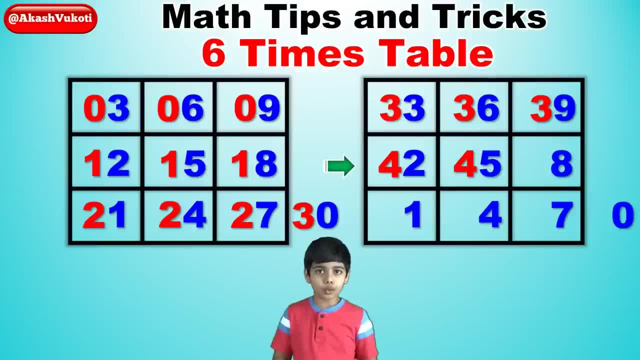 Yeah, you're pretty much right. It's 4,, 4, 4.. And for the tens digits in the bottom row of the second grid, we write 5,, 5, 5.. And then we write a 6. 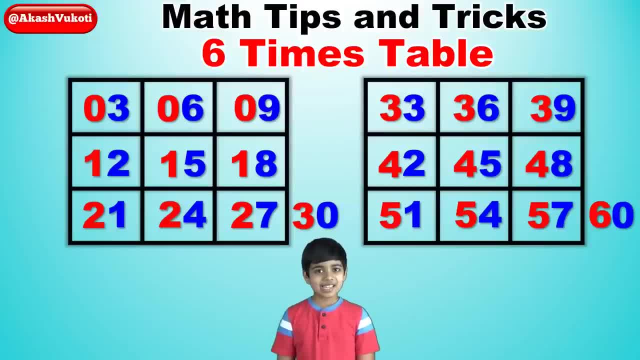 next to the second of two 0s. It sounds like a lengthy process, but you may actually notice that this is the 3 times table, from 3 times 1 to 3 times 20.. So if you know that, then well. 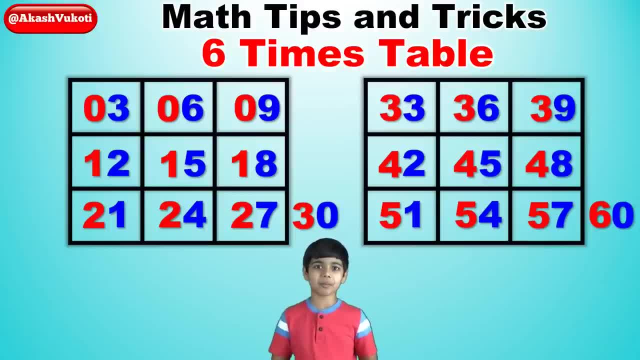 you kind of know the 6 times table using this trick. So now we can start. All you have to do is make a diamond shape in both of them and then connect the first diamond to the 30 and the second diamond to the 60.. 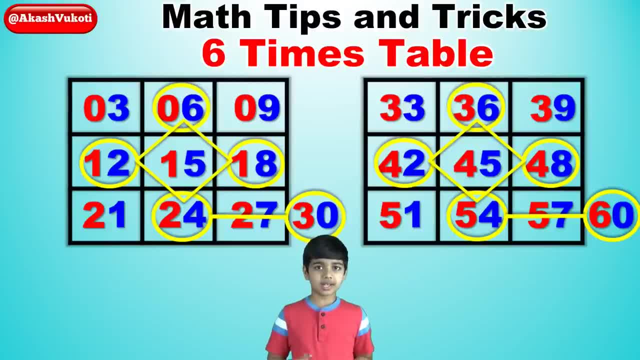 And make sure you circle all of these numbers that this diamond shape touches And all of the circled numbers create the 6 times table. Check this out. This thing is really cool. It's a really awesome trick. Yeah, this is amazing. 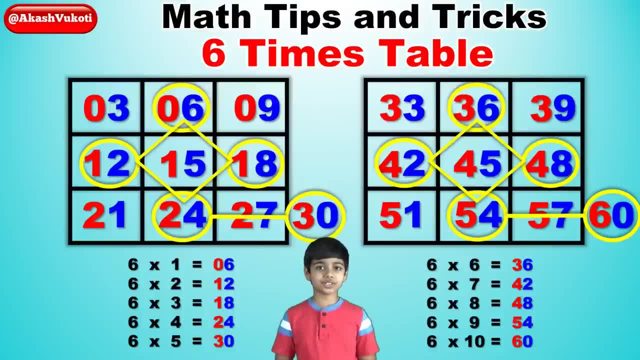 You can see behind me over there, we got the full 6 times table. It's a really awesome trick, in my opinion, really awesome. So now you know the trick to learning the 6 times table. You can use this trick. 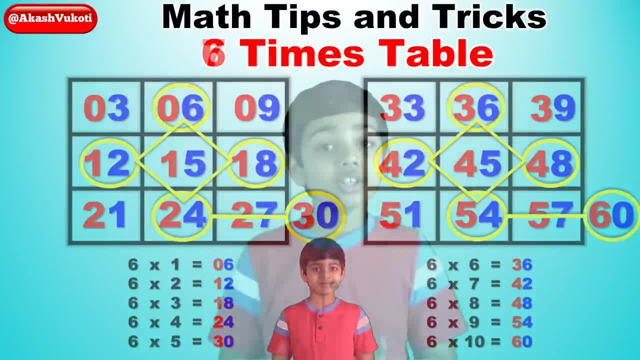 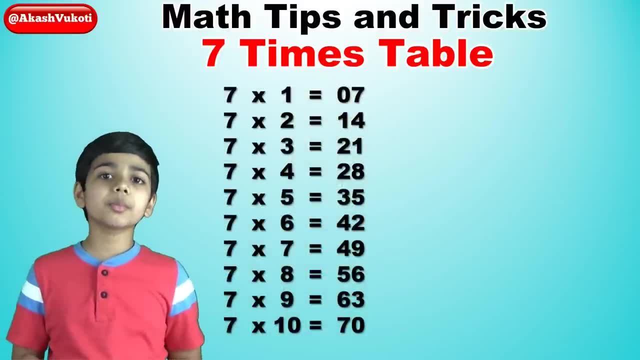 to memorize the 6 times table. We're going to learn the math trick for the 7 times table. Now let's begin by drawing out a 3 by 3 tic-tac-toe grid. as you can see behind me, 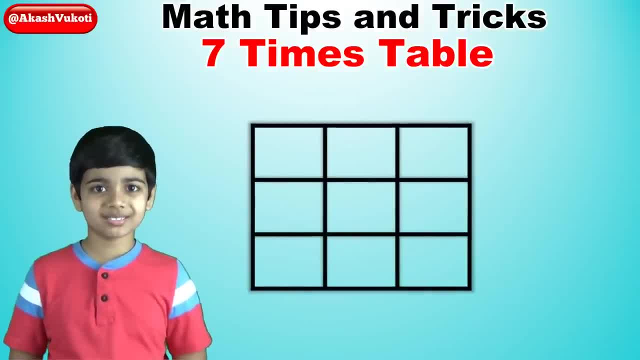 Now we can begin learning the trick For the ones digits. we go all the way to the top right box And write down the numbers from 1 to 9, by starting in the rightmost column and going back over to the leftmost column. 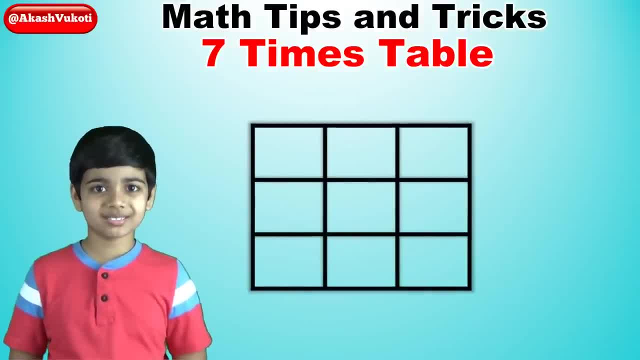 Now we can begin learning the trick For the ones digits. we go all the way to the top right box And write down the numbers from 1 to 9, by starting in the rightmost column and going back over to the leftmost column. 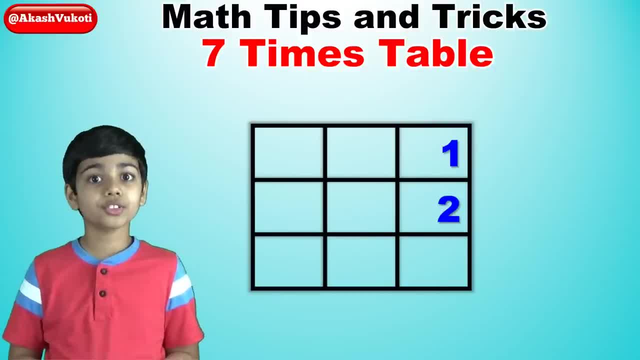 So 1,, 2,, 3,, 4,, 5,, 6,, 7,, 8,, 9.. And then you may be thinking: well, where's the 0?? So we write the 0 to the right of the bottom row. 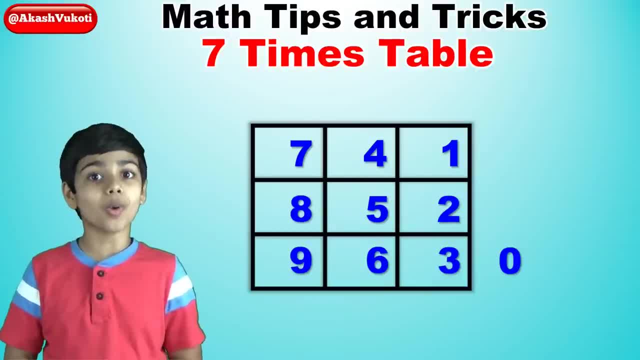 right here And that is the ones digits. Yep, we used up all of the digits And that is the ones digits of the 7 times table. Now we come to the tens digits. It's a little bit more complex, So we're going to break this up. 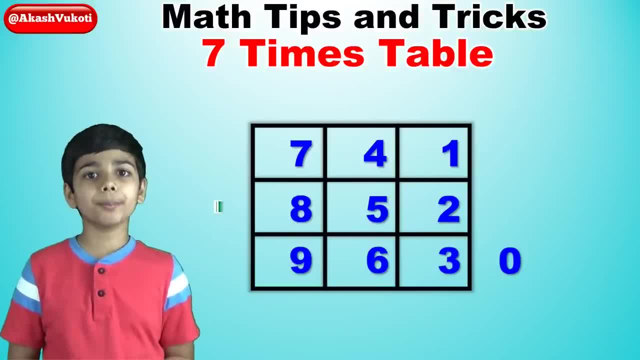 into three sections: Top row, middle row, bottom row. For the tens digits in the top row we will write 0 in the first box, 1 in the second box and 2 in the third box. OK for the tens digits. 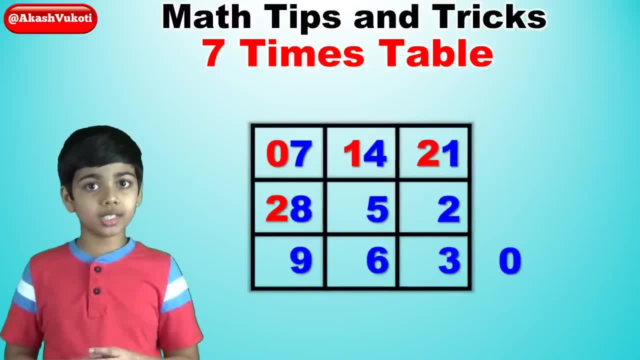 in the middle row, we will write 2 in the first box, 3 in the second box and 4 in the third box. And finally, for the tens digits in the bottom row, we will write 4 in the first box. 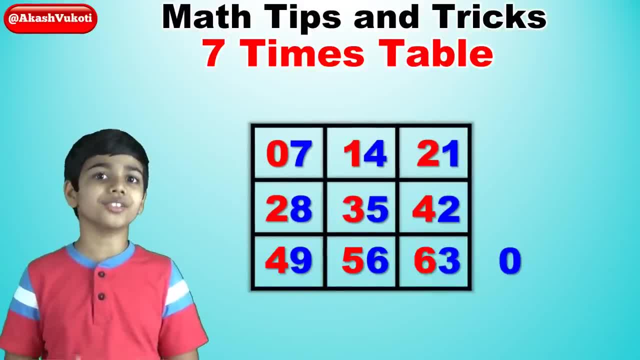 5 in the second box and 6 in the third box, And then to continue the line over to the 0,, we will write a 7 next to the 0 to get 70. And now you have the 7 times table. 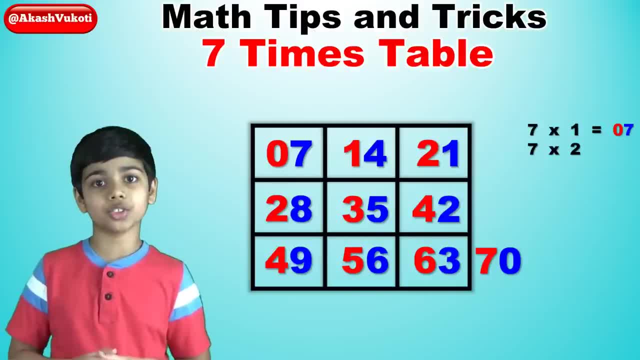 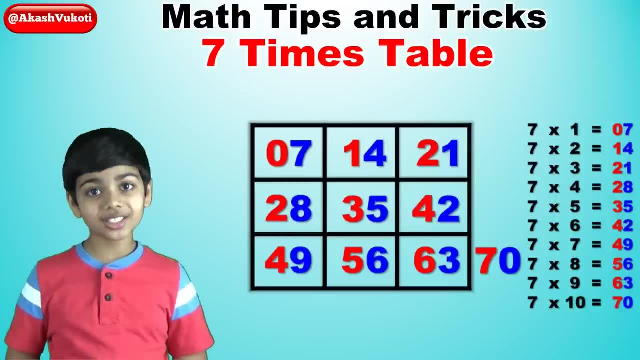 Take a look. This is a really, really, really awesome trick that will easily help you to memorize the 7 times table. So now you know the trick to learning the 7 times table, You can use it to start memorizing and putting into your brain. 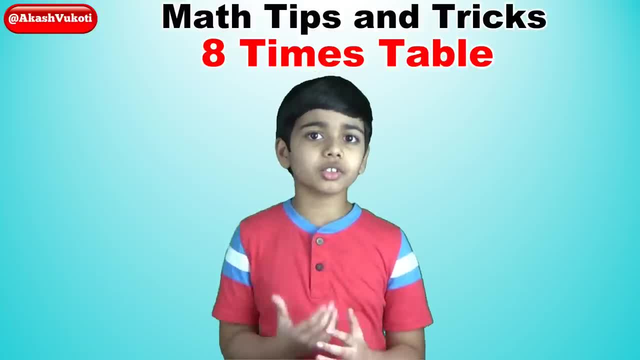 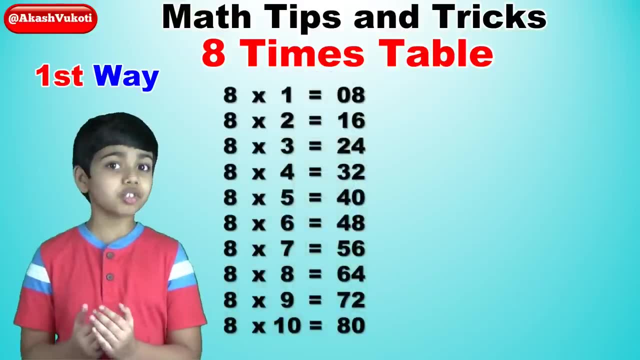 the 7 times table. For me, the most difficult multiplication table after the 9 times table is the 8 times table. Now here's the first way of explaining the trick. As this is the 8 times table, write down all of the numbers. 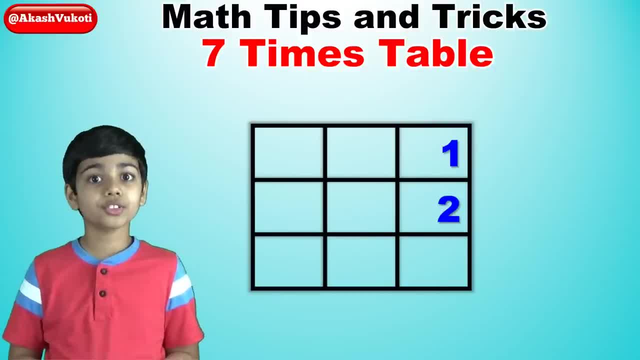 So 1,, 2,, 3,, 4,, 5,, 6,, 7,, 8,, 9.. And then you may be thinking: well, where's the zero? So we write the zero to the right of the bottom row. 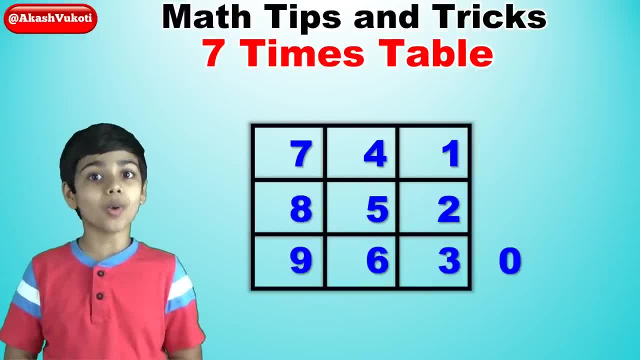 right here And that is the ones digits. Yep, we used up all of the digits And that is the ones digits of the 7 times table. Now we come to the tens digits. It's a little bit more complex, So we're going to break this up. 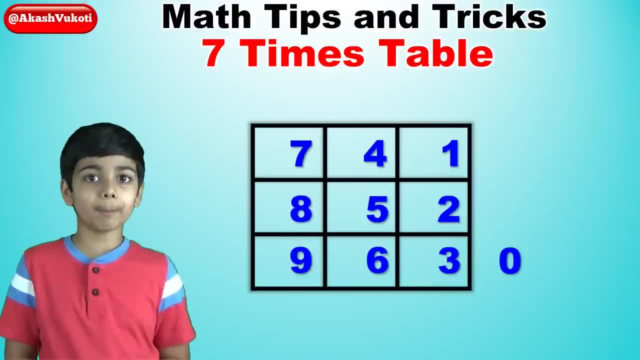 into three sections: Top row, middle row, bottom row. For the tens digits in the top row we will write zero in the first box, one in the second box and two in the third box. Okay, for the tens digits in the middle row. 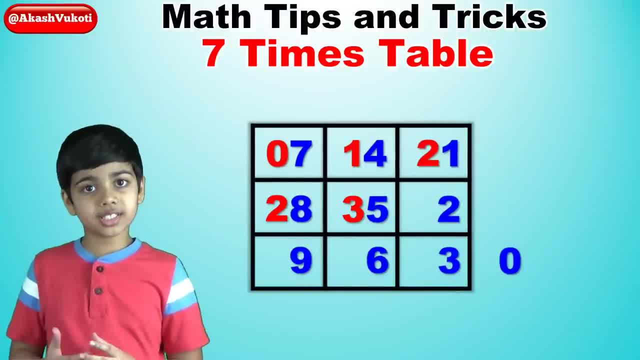 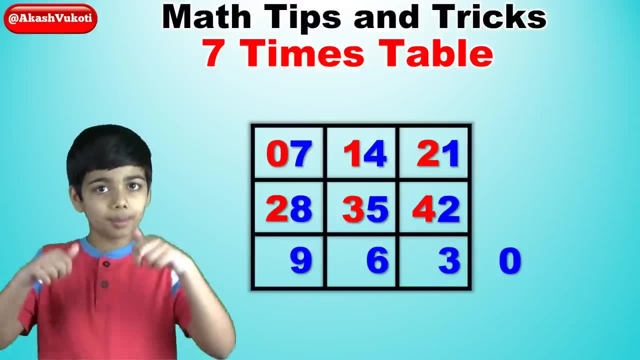 we will write two in the first box, three in the second box and four in the third box. And finally, for the tens digits in the bottom row, we will write four in the first box, five in the second box and six in the third box. 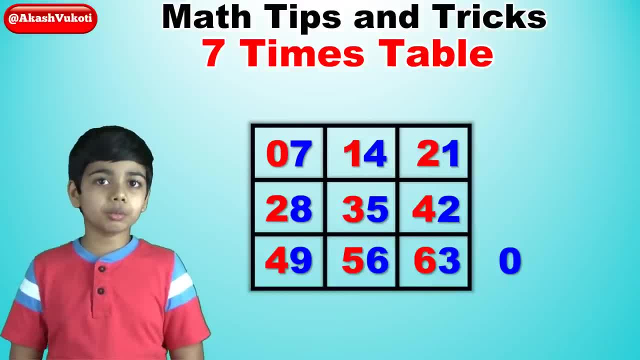 And then to continue the line over to the zero. we will write a seven to the zero to get 70. And now you have the seven times table. Take a look, This is a really, really, really awesome trick that will easily help you to memorize. 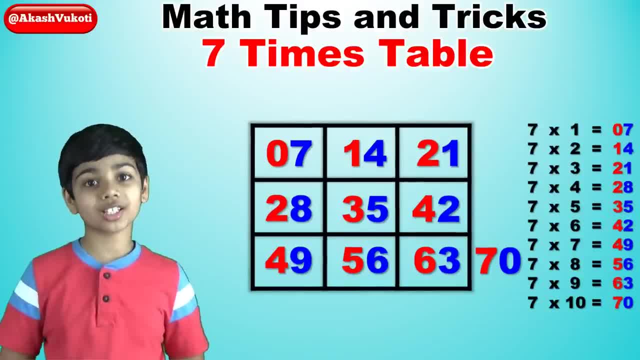 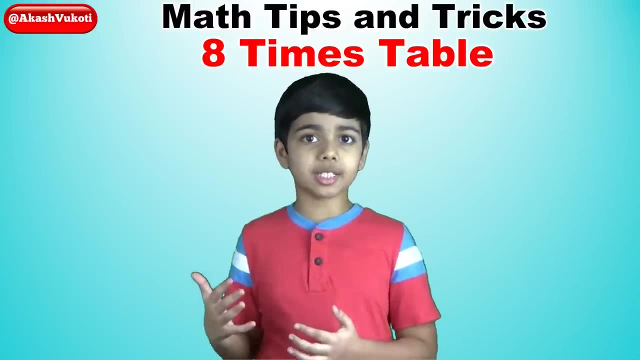 the seven times table. So now you know the trick to learning the seven times table. You can use it to start memorizing and putting into your brain the seven times table. For me, the most difficult multiplication table after the nine times table is the eight times table. 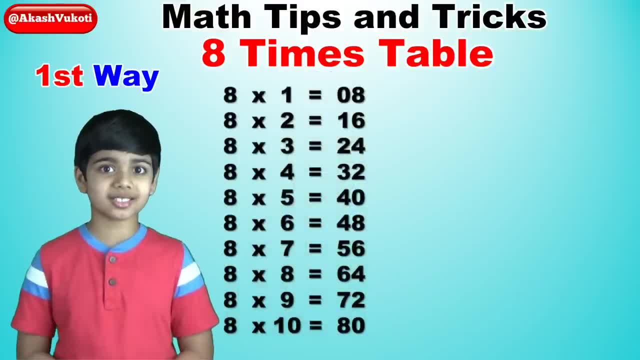 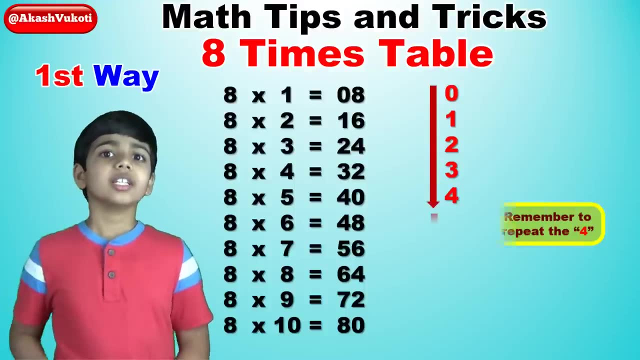 Now here's the first way of explaining the trick. As this is the eight times table, write down all of the numbers, from zero to eight, from top to bottom, as you're seeing behind me right here. But once you reach four, include an extra four. 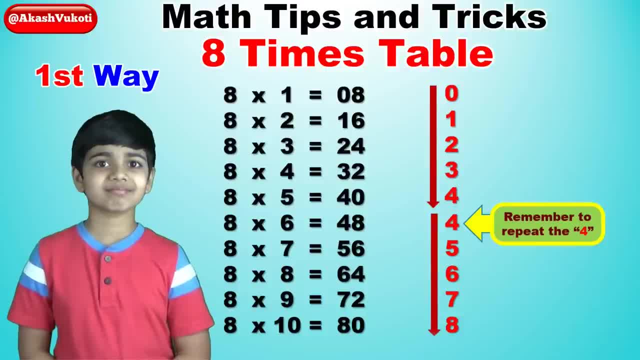 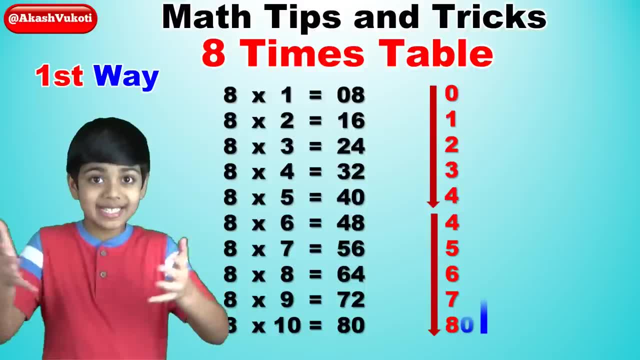 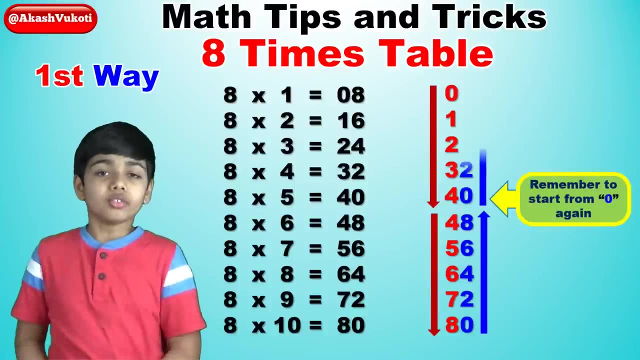 and continue until eight. Next, for the ones digits, write the two times table, starting from zero up to eight, again from bottom to top, And once you reach eight, repeat and go again from zero up to eight And once you're done, 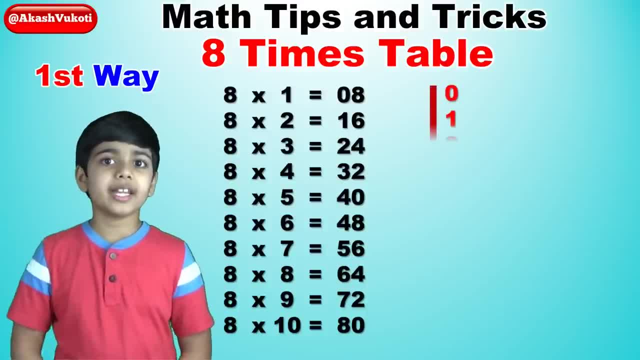 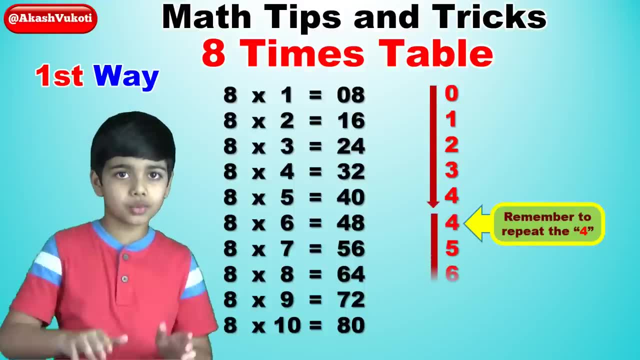 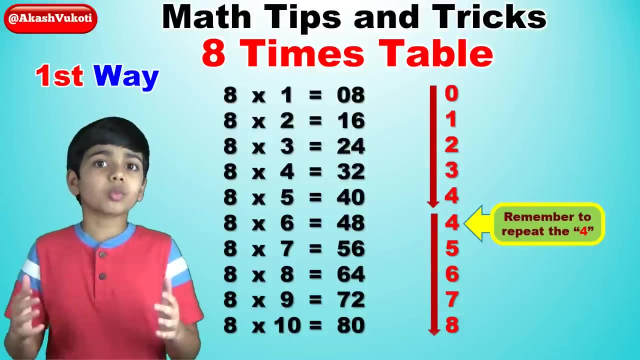 from 0 to 8, from top to bottom, as you're seeing behind me right here. But once you reach 4, include an extra 4 and continue until 8.. Next, for the ones digits, write the 2 times table. 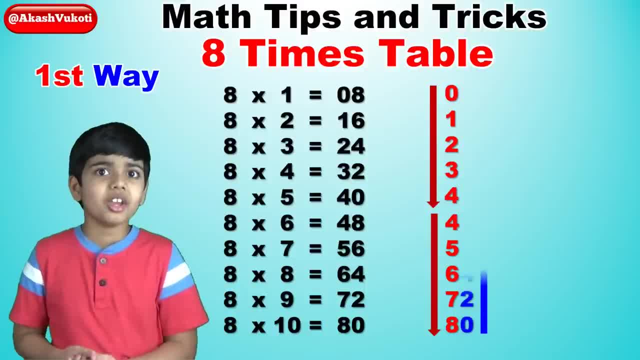 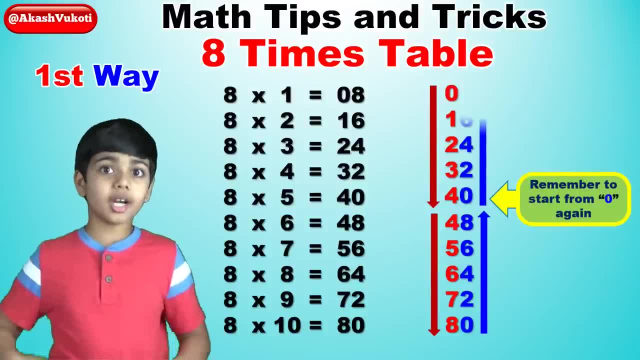 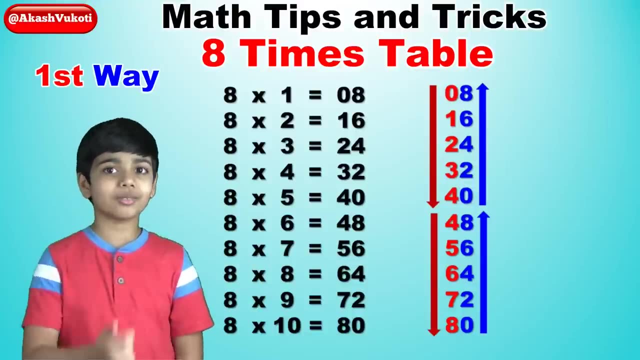 starting from 0 up to 8, again from bottom to top, And once you reach 8, repeat and go again from 0 up to 8. And once you're done, you have the 8 times table, as you can see right here. 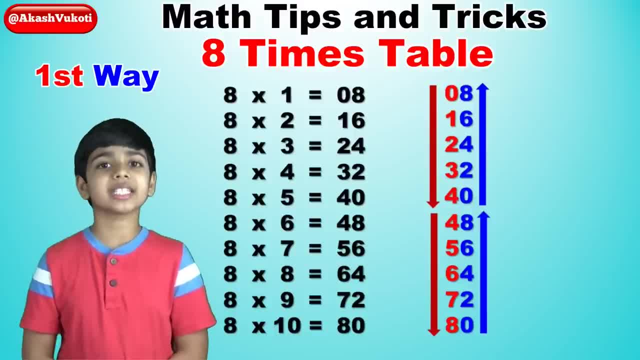 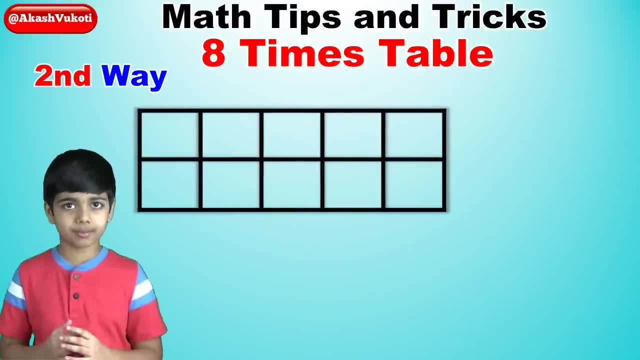 And here is the second way of explaining the trick, As you can see here, let's create a box of 5 columns and 2 rows For the ones digits, just like you've seen in the first method we're going to write down. 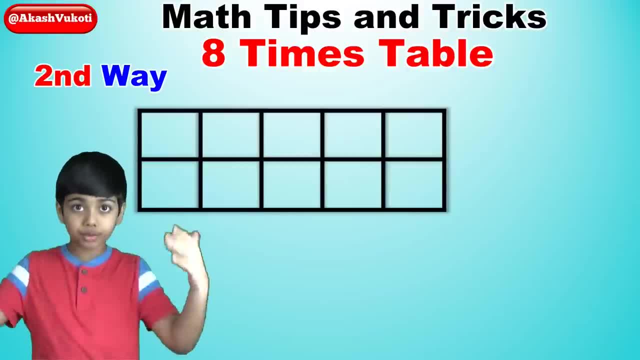 the 2 times table: from 0 to 8 in both rows, but this time backwards, in the opposite direction. from 8 to 0. So 8,, 6,, 4,, 2, 0.. Now for the tens digits. 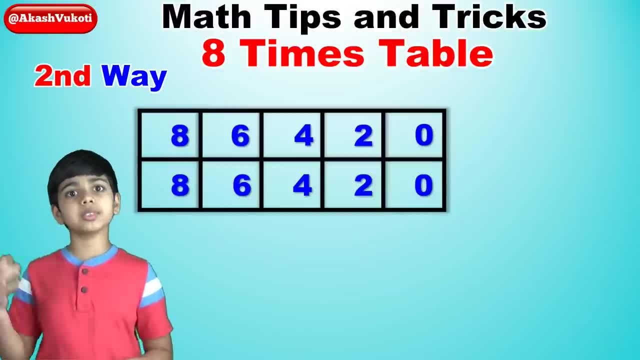 in the first row, we will write down the numbers from 0 to 4, as you see here, And for the tens digits in the second row, we will write the numbers from 4 to 8.. And once you're finished, 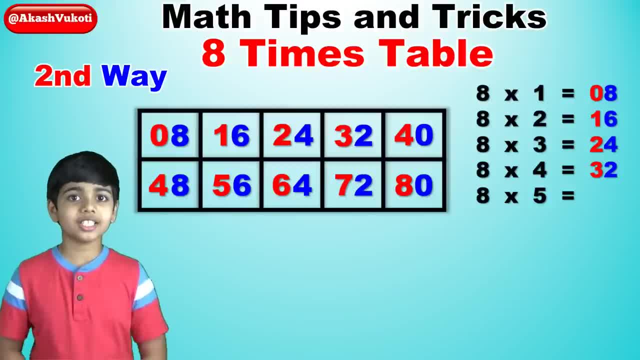 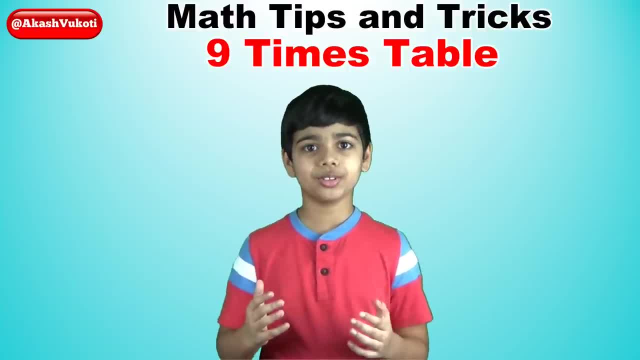 you will have the 8 times table, as you can see right here. Do you know the 9 times table? I'm sure you do, But for me the 9 times table is the hardest one out of all the multiplication tables from 1 to 9.. 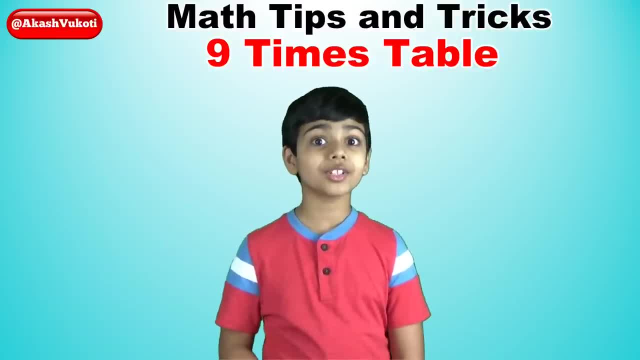 But recently I found not 1,, not 2,, not 3, but 4 simple tricks to easily remember the 9 times table. I'll let you know about these in today's video Once you've mastered these easy tricks. 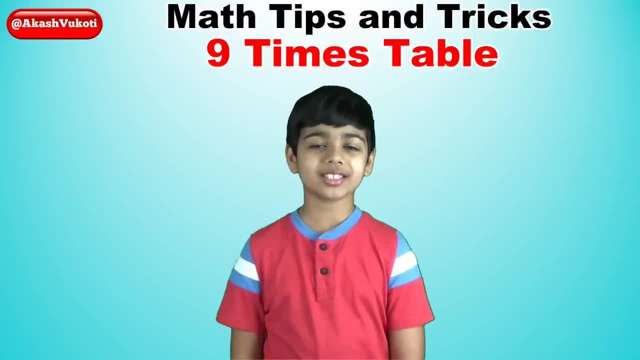 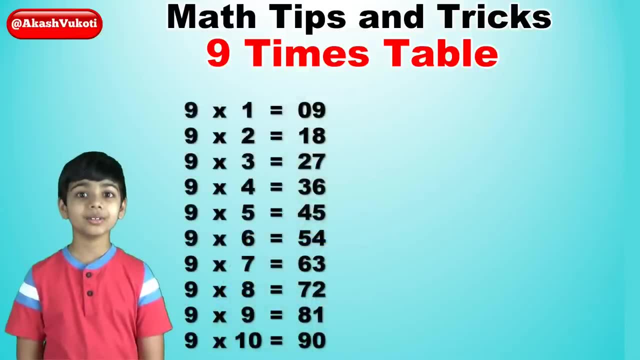 you will easily agree with me that the 9 times table is indeed the easiest multiplication table. Now I'm going to tell you how special the 9 times table is, So let's take a closer look. The first specialty is that, if you look carefully, 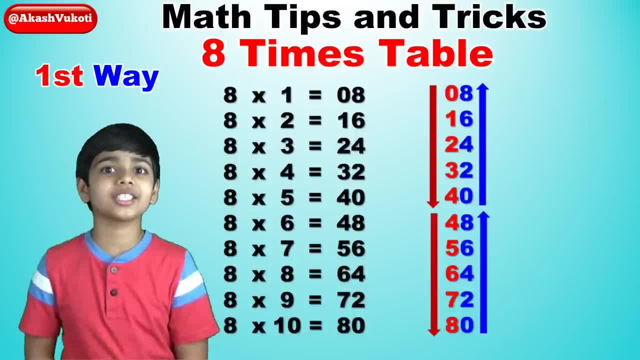 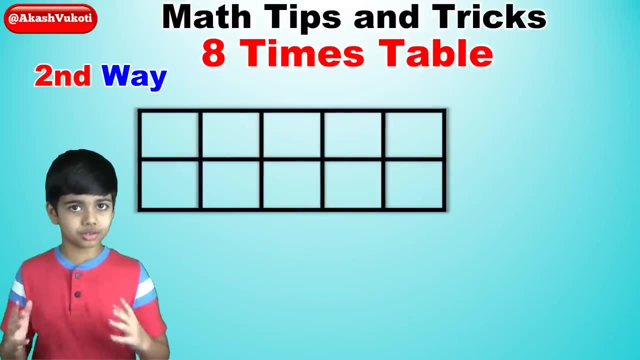 you have the eight times table, as you can see right here. And here is the second way of explaining the trick. As you can see here, let's create a box of five columns in two rows For the ones digits, just like you've seen in the first method. 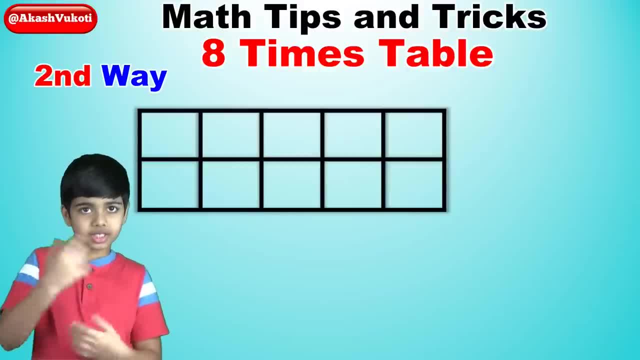 we're going to write down the two times table: from zero to eight in both rows, but this time backwards, in the opposite direction, from eight to zero. So eight, six, four, two, zero. Now for the tens digits in the first row. 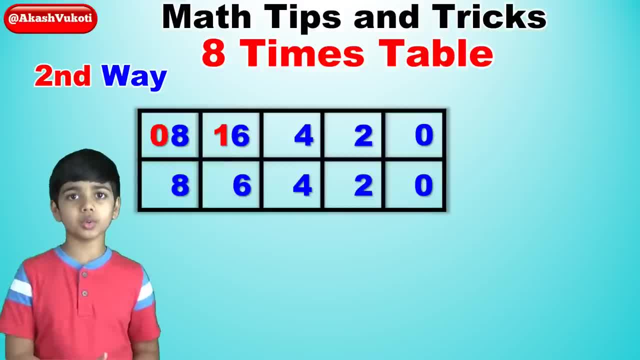 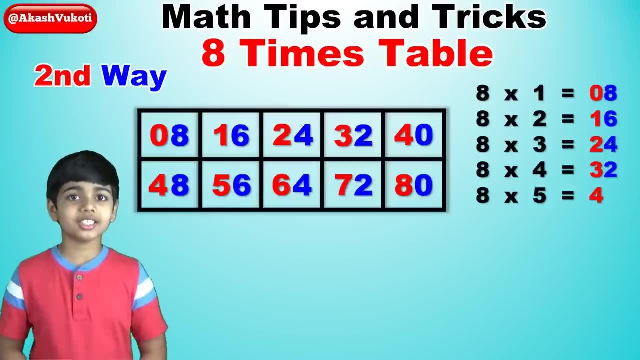 we will write down the numbers from zero to four, as you see here, And for the tens digits in the second row we will write the numbers from four to eight And once you're finished you will have the eight times table, as you can see right here. 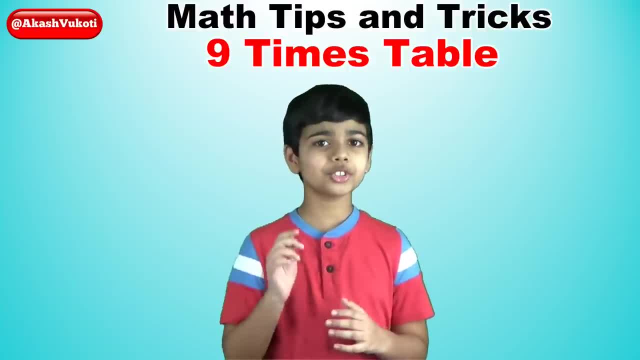 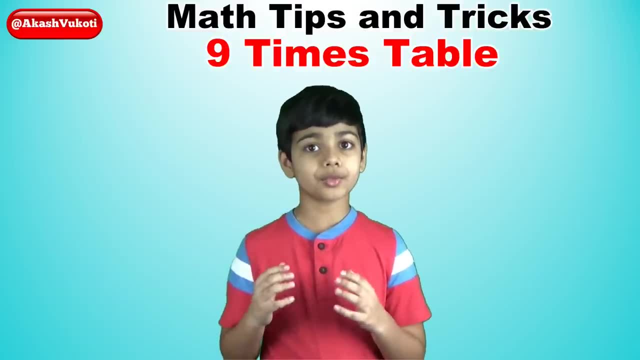 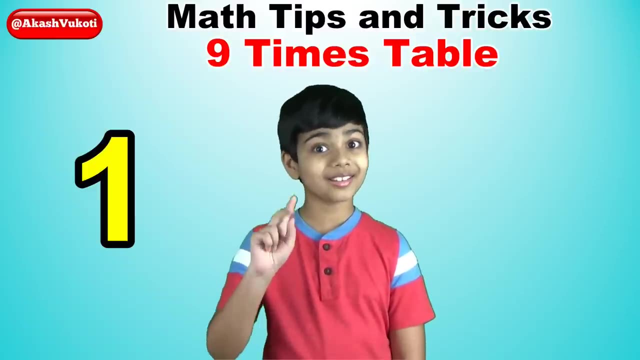 Do you know the nine times table? I'm sure you do, But for me the nine times table is the hardest one out of all the multiplication tables from one to nine. But recently I found not one, not two, not three. 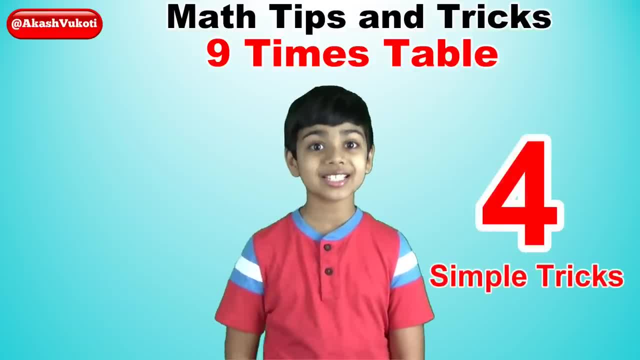 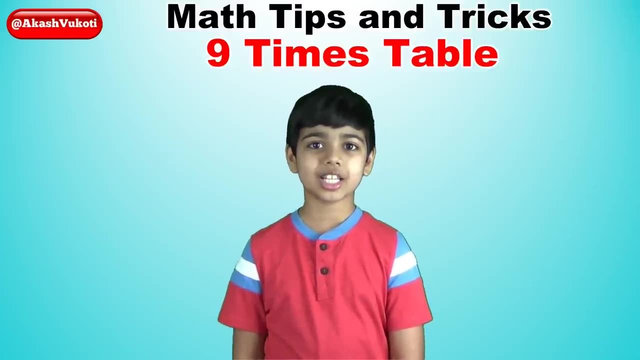 but four simple tricks to easily remember the nine times table. I'll let you know about these in today's video. Once you've mastered these easy tricks, you will easily agree with me that the nine times table is indeed the easiest multiplication table. Now. 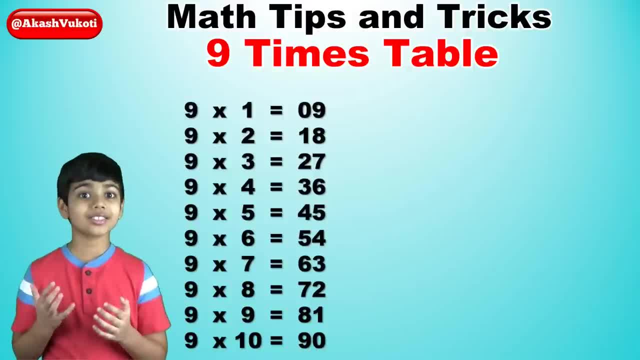 I'm going to tell you how special the nine times table is. So let's take a closer look. The first specialty is that, if you look carefully, all of the products of the nine times table can be read as two columns: The left column. 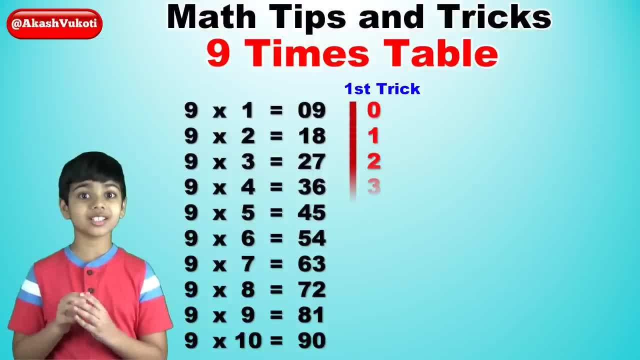 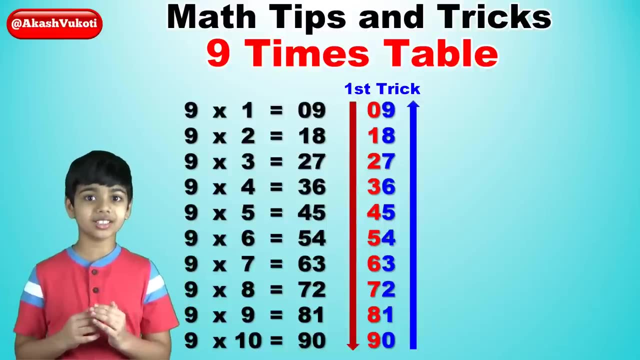 has all the numbers from zero to nine in ascending order, And the right column has all the numbers in reverse order, from nine to zero. as you can see right here, The second trick is that the sum of the digits of each answer is nine. 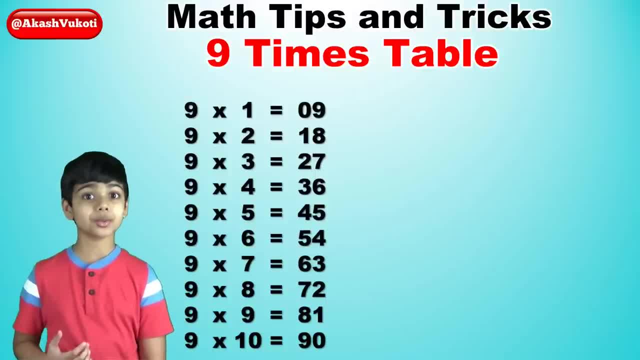 all of the products of the 9 times table can be read as two columns. The left column has all the numbers from 0 to 9 in ascending order, And the right column has all the numbers in reverse order, from 9 to 0,. 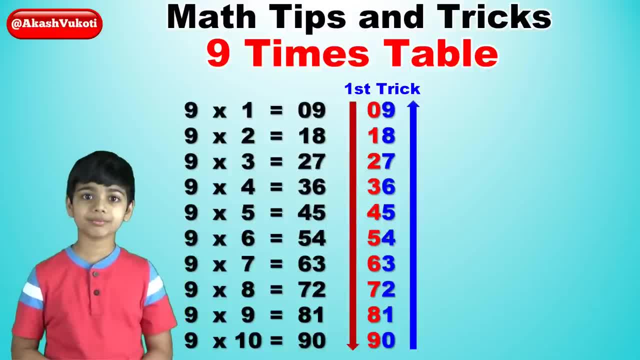 as you can see right here, The second trick is that the sum of the digits of each answer is 9.. So, as you can see here, 0 plus 9 is 9.. 1 plus 8 is 9.. 2 plus 7 is 9.. 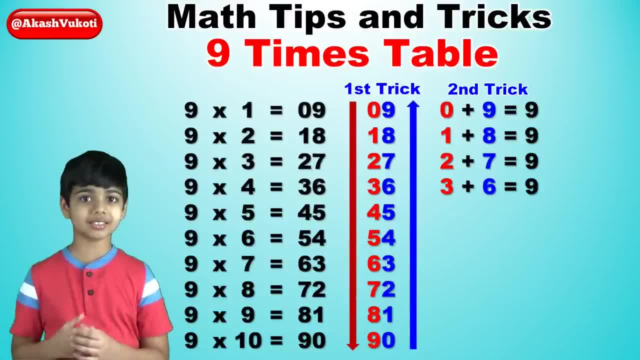 3 plus 6 is 9.. 4 plus 5 is 9.. 5 plus 4 is 9.. 6 plus 3 is 9.. 7 plus 2 is 9.. 8 plus 1 is 9.. 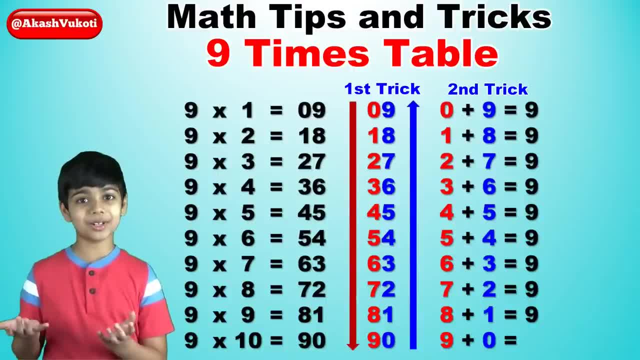 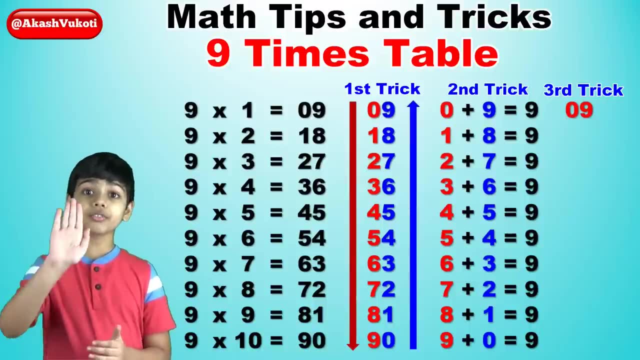 And finally, 9 plus 0 is well 9.. The third trick is that you'll notice that 9 times 1 is 0,, 9, or 9,, and 9 times 10 is the reverse: 9, 0,. 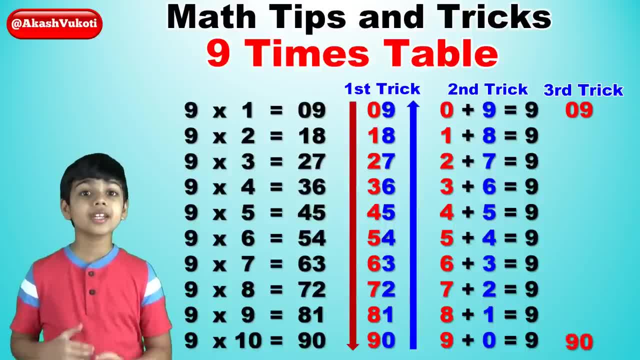 or 90.. In the same way, 9 times 2 is 18, and 9 times 9 is 81.. 9 times 3 is 27, and 9 times 8 is 72.. 9 times 4: 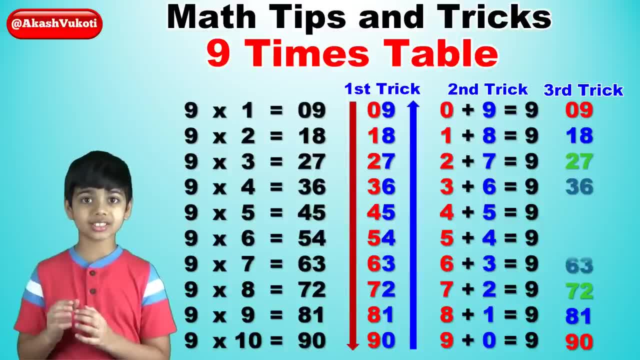 is 36, and 9 times 7 is 63.. And finally, 9 times 5 is 45, and 9 times 6 is 54.. These are three super easy tricks to memorize the 9 times table. 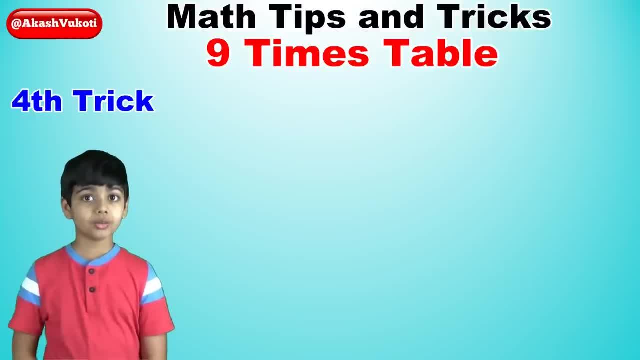 However, there is the fourth trick, which is the quickest and fastest and easiest way to remember the 9 times table. Here it is: Say you want to multiply 9 times 4.. What you have to do is take that number 4. 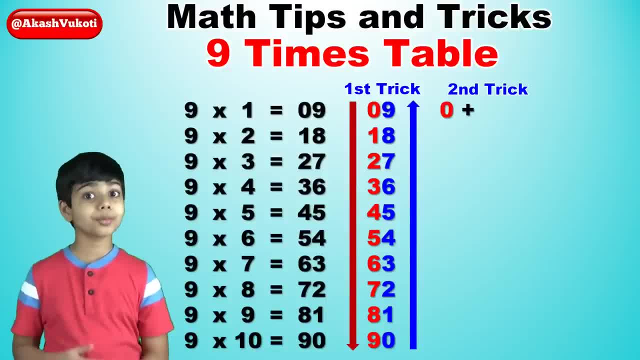 So, as you can see here, zero plus nine is nine. One plus eight is nine. Two plus seven is nine. Three plus six is nine. Four plus five is nine. Five plus four is nine. Six plus three is nine. Seven plus two is nine. 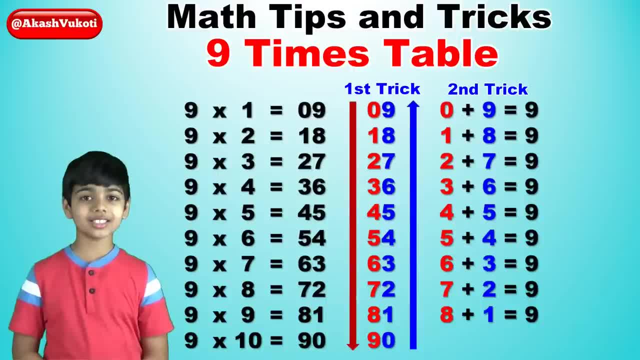 Eight plus one is nine And finally, nine plus zero is well nine. The third trick is that you'll notice that nine times one is zero, nine or nine, And nine times ten is the reverse: nine, zero or ninety. In the same way, 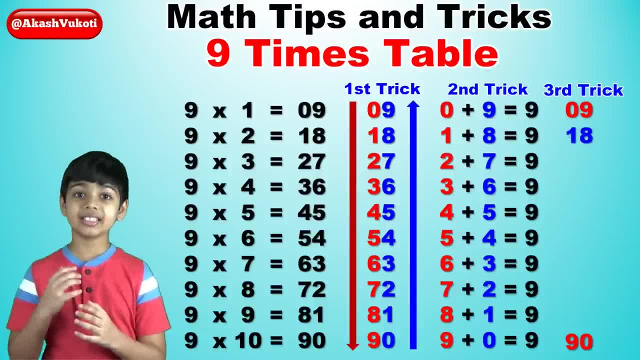 nine times two is eighteen, and nine times nine is eighty-one. Nine times three is twenty-seven and nine times eight is seventy-two. Nine times four is thirty-six and nine times seven is sixty-three. And finally, nine times five is forty-five. 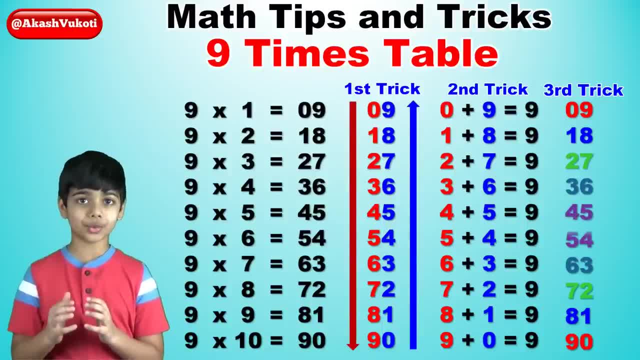 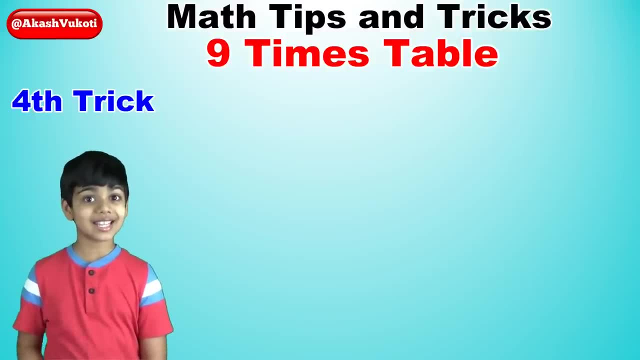 and nine times six is fifty-four. These are three super easy tricks to memorize the nine times table. However, there is the fourth trick, which is the quickest and fastest and easiest way to remember the nine times table. Here it is: Say you want to multiply. 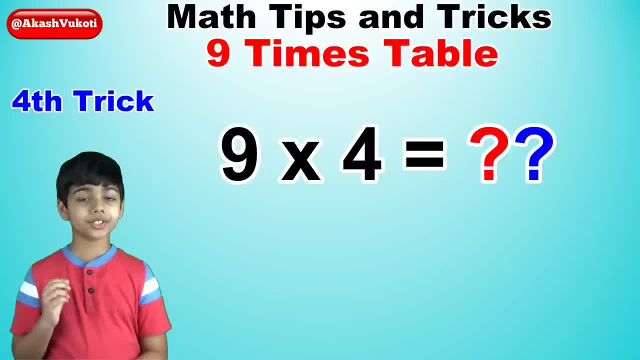 nine times four. What you have to do is take that number four and find the number before it, which in this case is three. This number is the first digit. The last digit is found by subtracting this number from nine. So nine minus three is six. 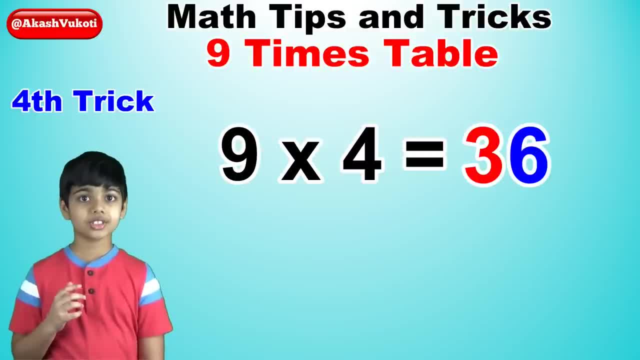 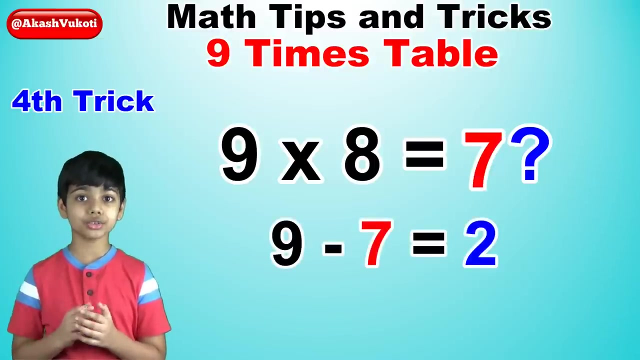 Six is the last digit. So three is the first digit, Six is the last digit. The answer is thirty-six. Let's take another example. Say nine times eight, The number before eight is seven, which is the first digit. Nine minus seven is two. 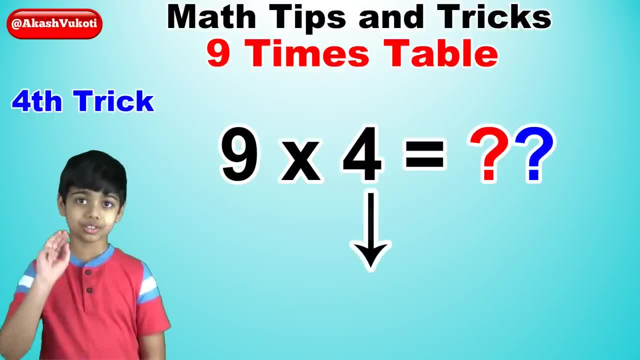 and find the number before it, which in this case is 3.. This number is the first digit. The last digit is found by subtracting this number from 9.. So 9 minus 3 is 6.. 6 is the last digit. 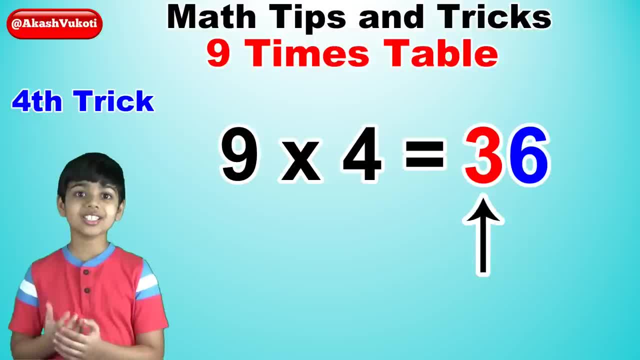 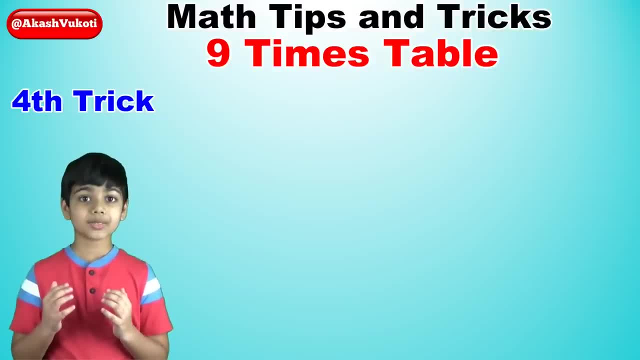 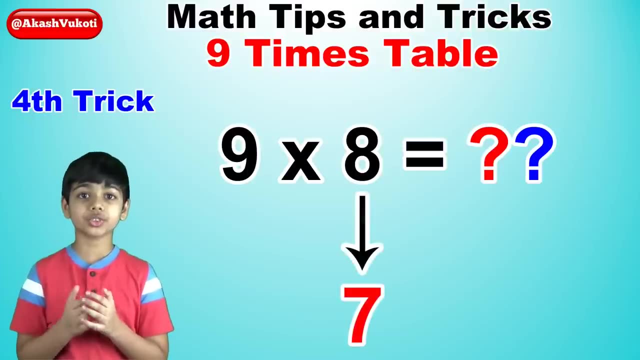 So 3 is the first digit, 6 is the last digit. The answer is 36.. Let's take another example. Say 9 times 8.. The number before 8 is 7,, which is the first digit. 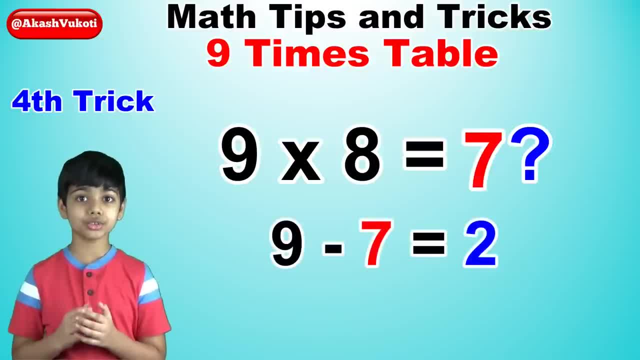 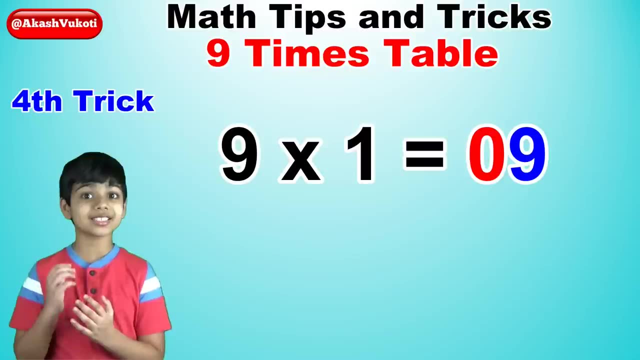 9 minus 7 is 2, which is the last digit. 7 is the first digit, 2 is the last digit. The answer is 72.. 9 times 1 is 9 and we all know that, because any number 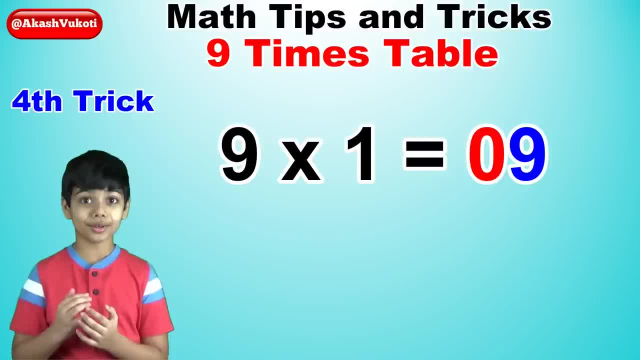 times 1 is that number, But did you know that it applies here too? The number before 1 is 0, and 9 minus 0 is well 9.. So 09 or 9 is the answer. This. 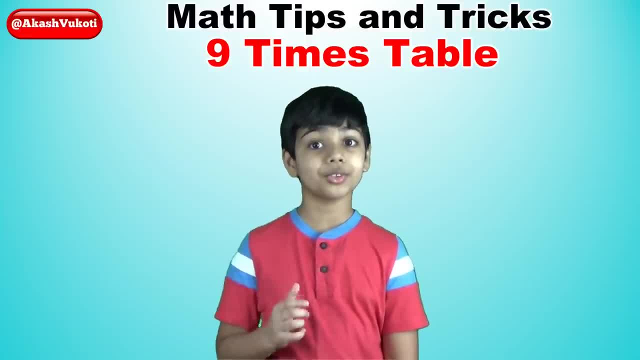 is the best trick to remember the 9 times table in your brain without using a pen and paper and, of course, a calculator. I'm very sure that this trick will help you whenever you need the 9 times table, Like in class. 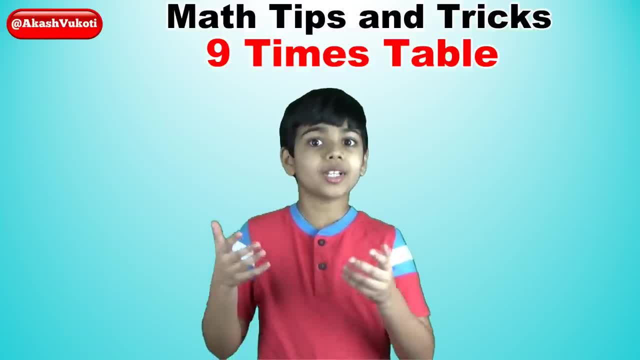 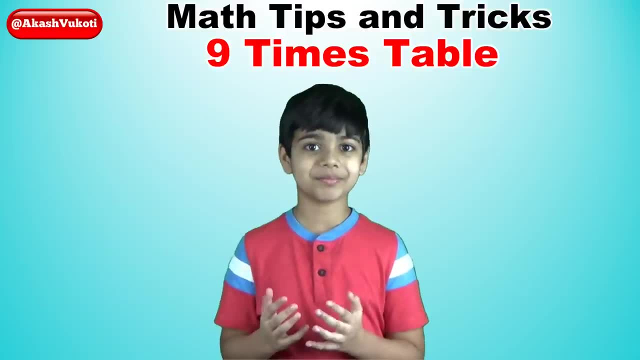 or in your exam, or if someone asks you let's say what's 9 times 7, you can just remember this trick and quickly say the answer is 63.. So that's about it. Hello friends, I'm Akash. 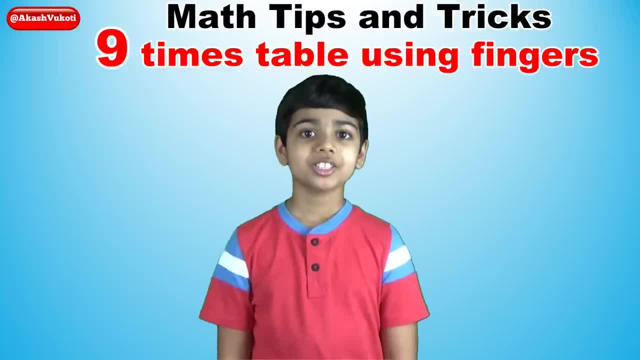 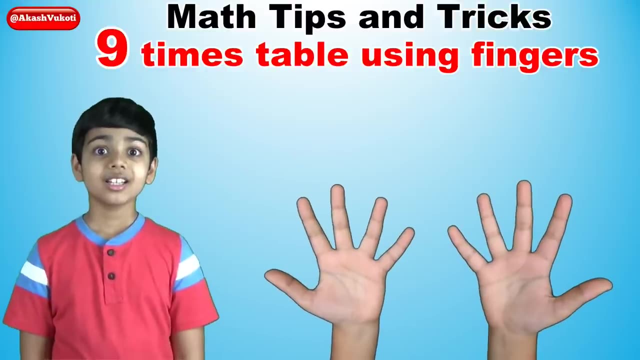 Today, I want to show you the best way to remember the 9 times table using only your hands or fingers. So let's begin by opening up both hands in front of you like this: Now imagine that your fingers represent the numbers 1 through 10.. 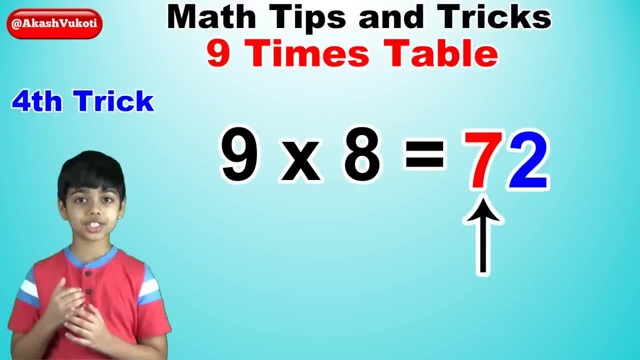 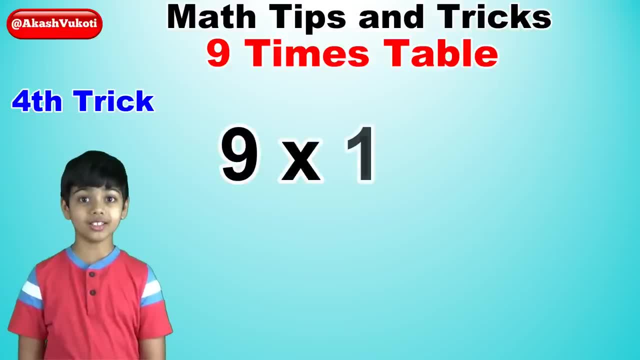 which is the last digit. Seven is the first digit. Two is the last digit. The answer is seventy-two Nine times one is nine, and we all know that, because any number times one is that number. But did you know that it applies here too? 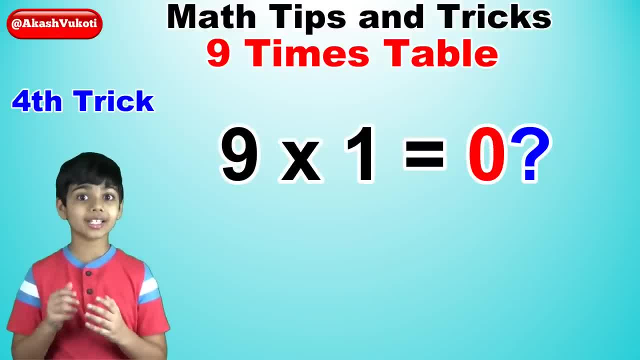 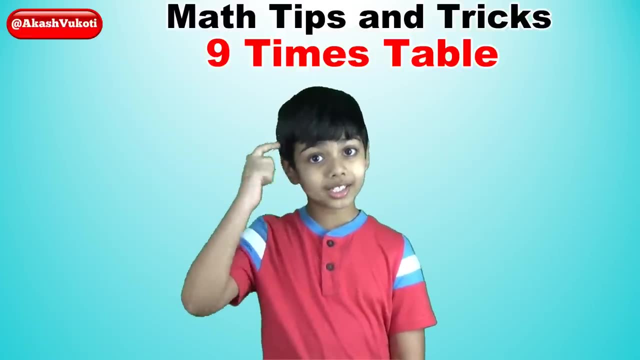 The number before one is zero, and nine minus zero is well nine. So zero-nine or nine is the answer. This is the best trick to remember the nine times table in your brain without using a pen and paper and, of course, a calculator. 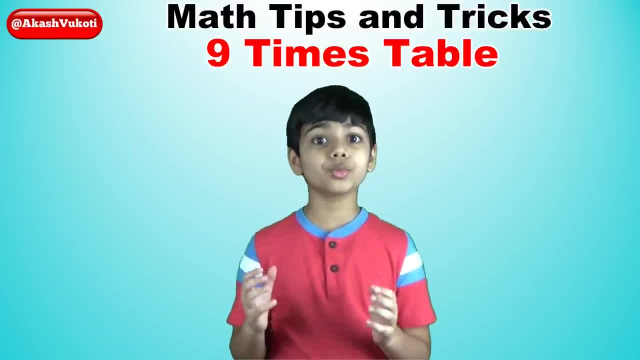 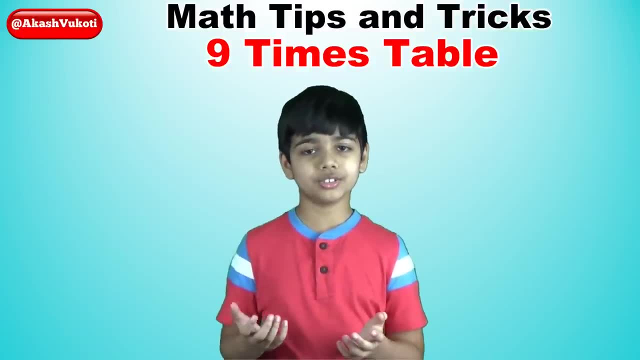 I'm very sure that this trick will help you whenever you need the nine times table, Like in class or in your exam, or if someone asks you let's say what's nine times seven. You can just remember this trick and quickly say the answer is sixty-three. 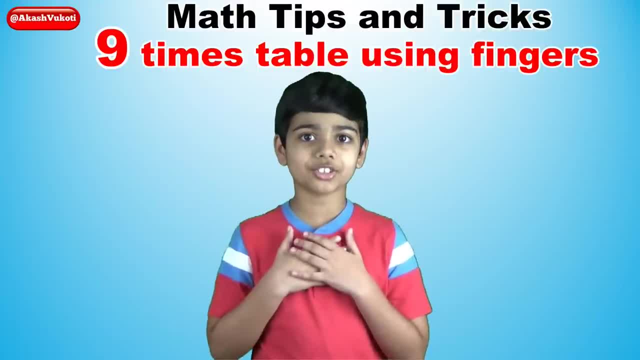 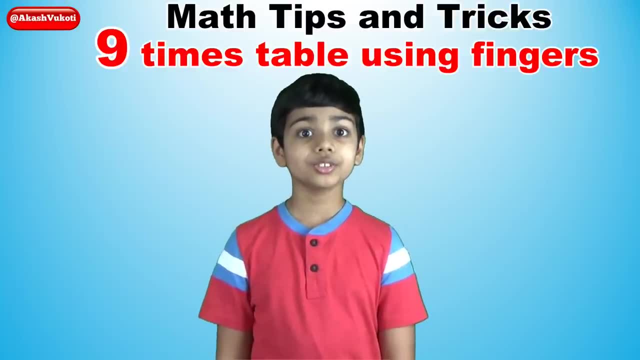 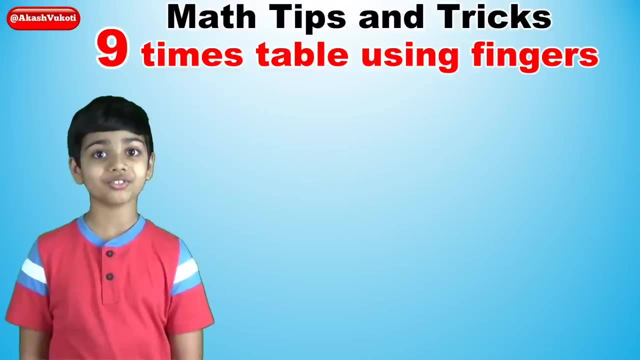 So that's about it. Hello friends, I'm Akash. Today, I want to show you the best way to remember the nine times table using only your hands or fingers, So let's begin by opening up both hands in front of you. 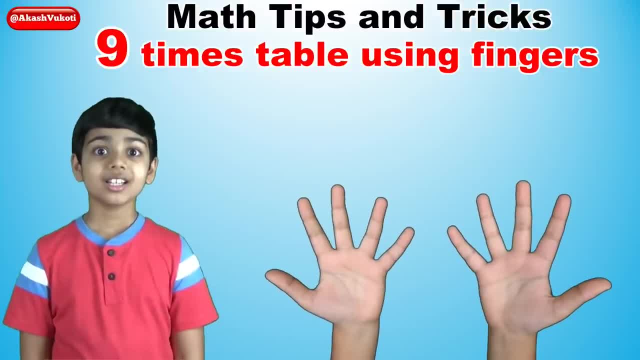 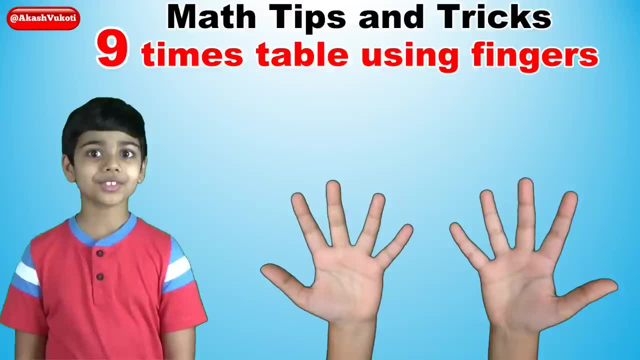 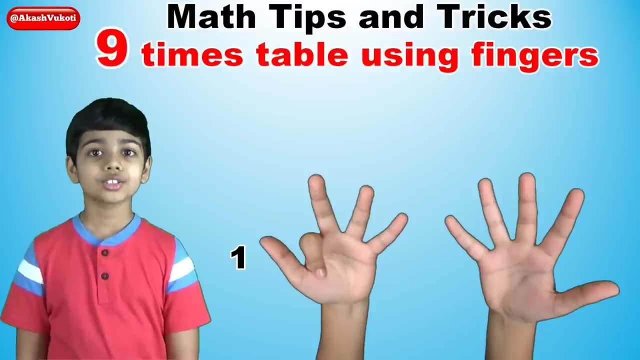 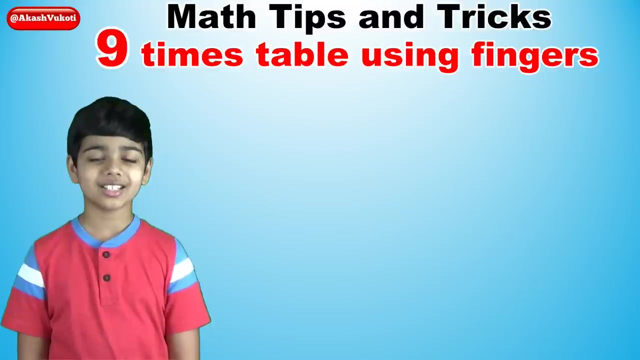 like this. Now imagine that your fingers represent the numbers one through ten. Your left thumb is the number one and your right thumb is the number ten. So one, two, three, four, five, six, seven, eight, nine, ten. 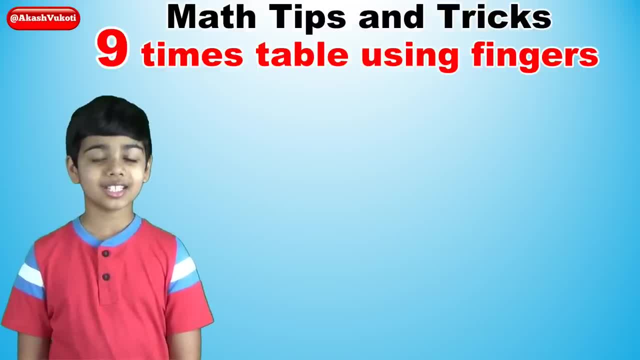 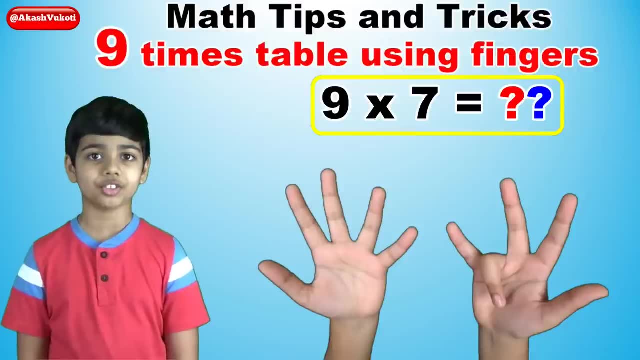 Now let's begin. Let's take an example. Say nine times seven. Let's start by folding the seventh finger down like this. You're seeing the answer right now. actually, There are six fingers to the left of the folded finger: seven. 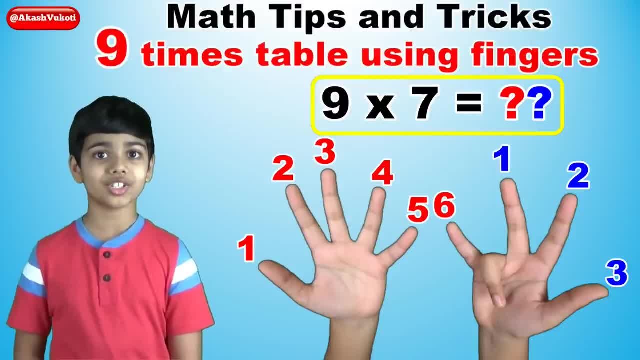 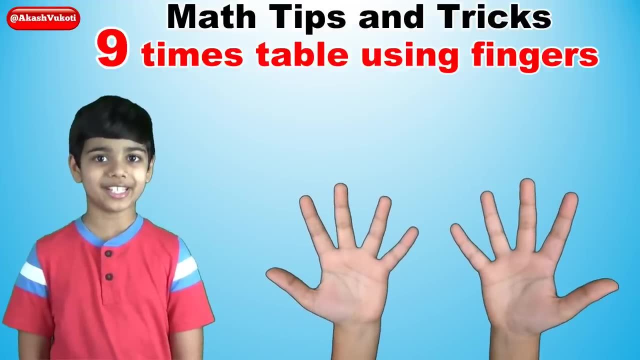 and there are three fingers to the right of the folded finger, So the answer is sixty-three. You're seeing it right now. It's a super nice trick. right Now let's do the nine times table from the very beginning. Nine times one. 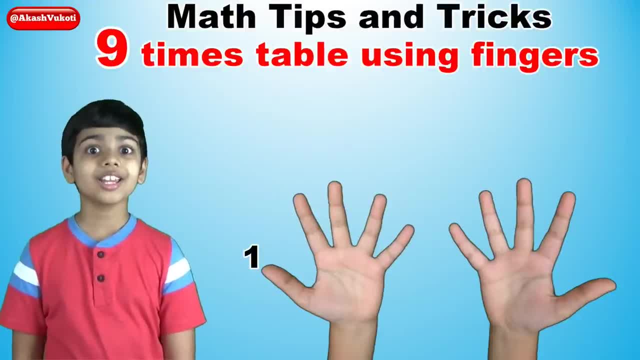 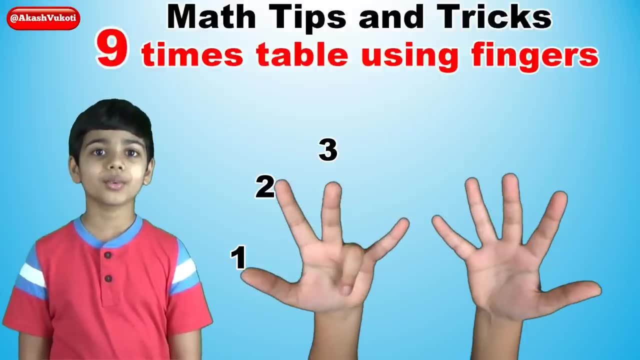 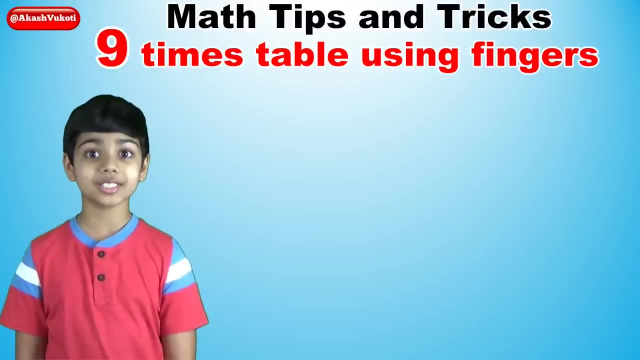 Your left thumb is the number 1 and your right thumb is the number 10.. So 1,, 2,, 3,, 4,, 5,, 6,, 7,, 8,, 9,, 10.. Now 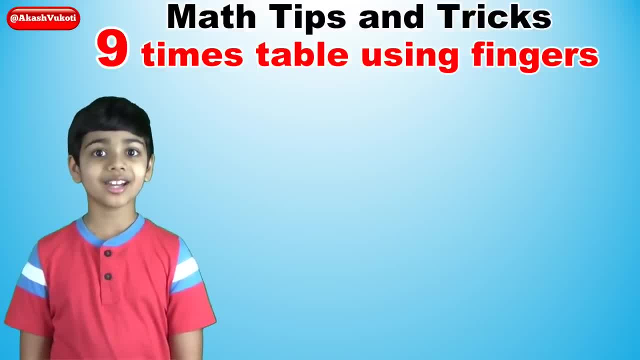 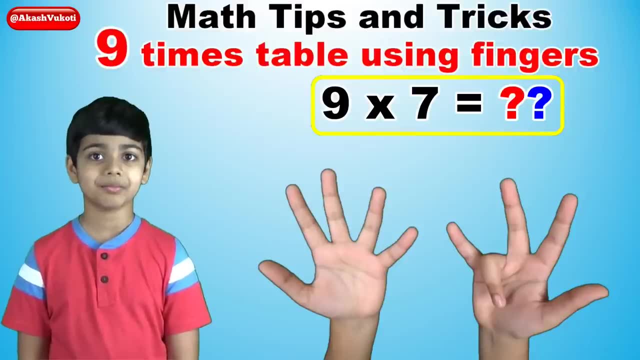 let's begin. Let's take an example. Say 9 times 7.. Let's start by folding the 7th finger down like this. You're seeing the answer right now. actually, There are 6 fingers to the left of the table. 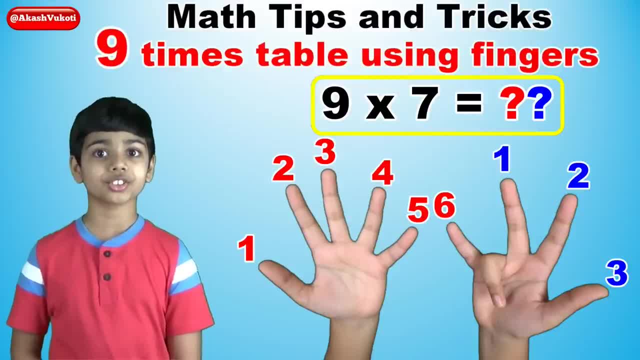 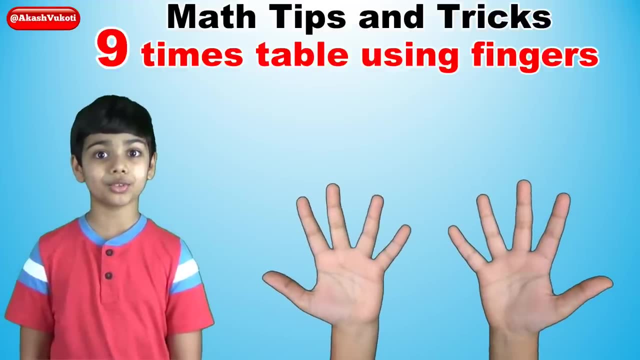 There are 6 fingers to the right of the folded finger, 7, and there are 3 fingers to the right of the folded finger. So the answer is 63.. You're seeing it right now. It's a super nice trick, right. 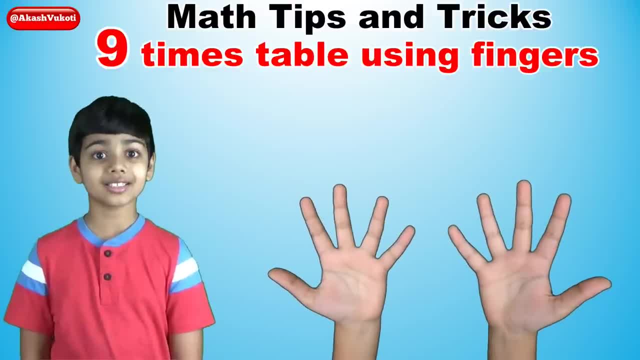 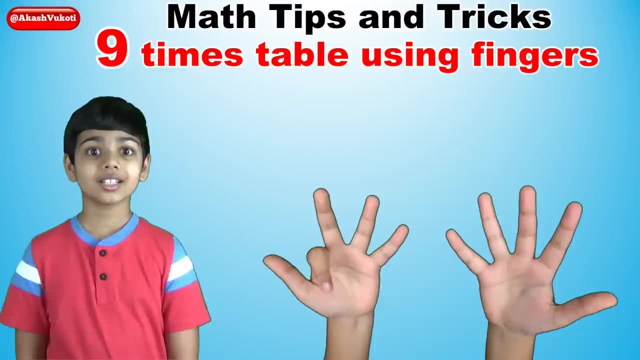 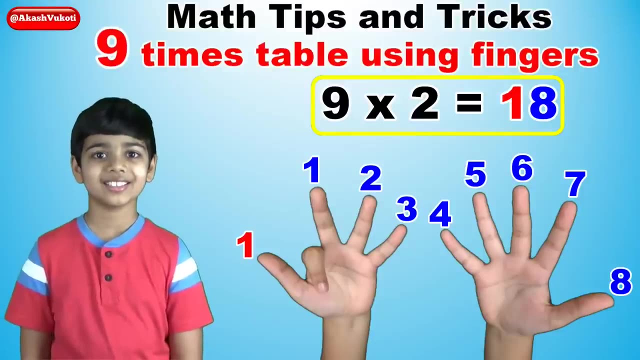 Now let's do the 9 times table from the very beginning. 9 times 1 is 0, 9,. 2, is 1, 8, 18.. 9 times 3 is 2, 7,. 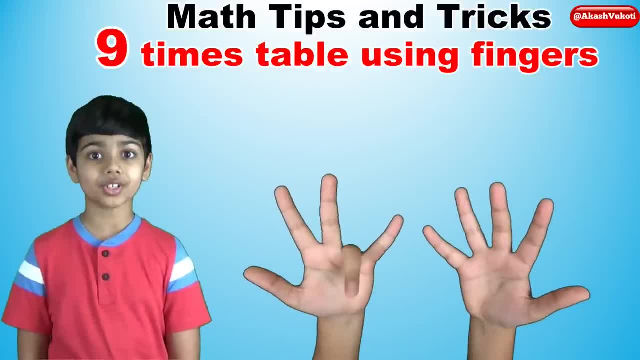 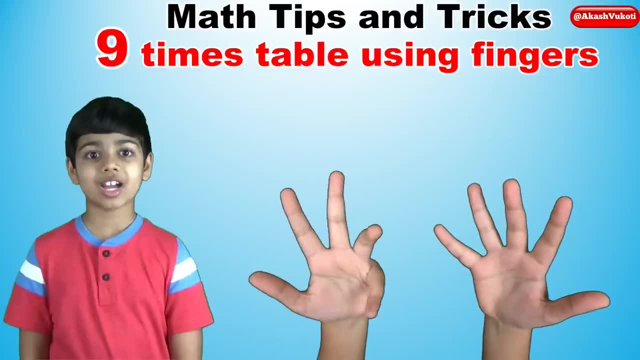 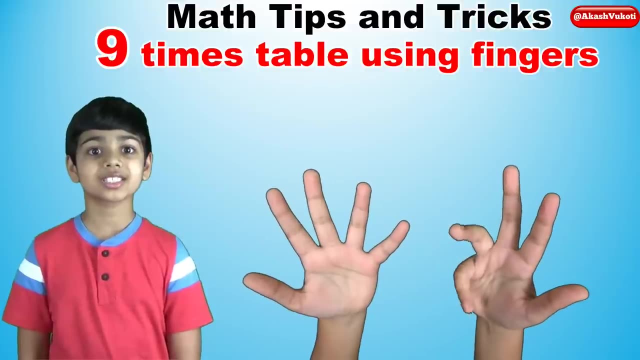 27. 9 times 4 is 3, 6,, 36.. 9 times 5 is 4, 5, 45.. 9 times 6 is 5, 4,, 54.. 9 times. 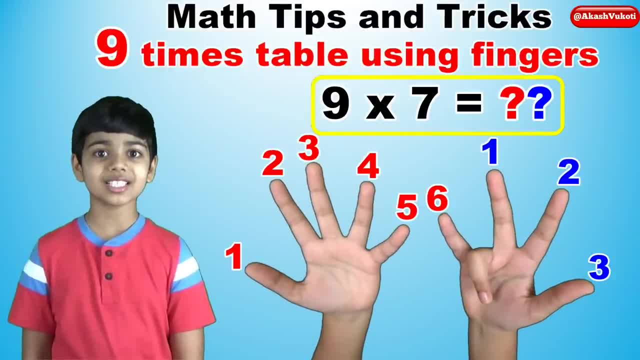 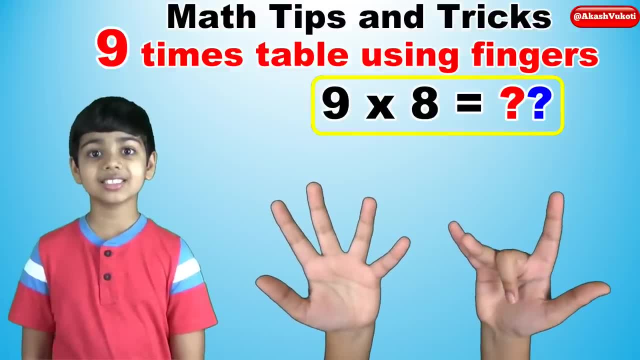 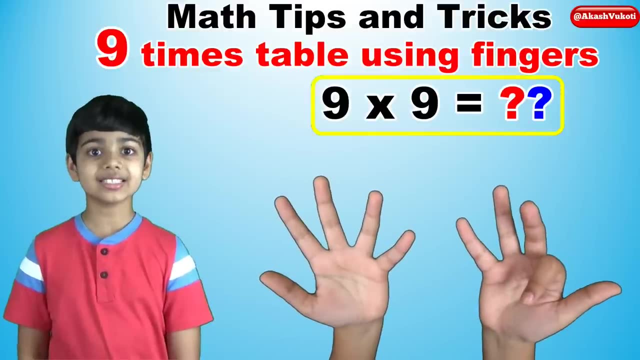 7 is 6, 3, 63.. 9 times 8 is 7, 2, 72.. 9 times 9 is 8, 1, 81.. And finally, 9 times 10 is. 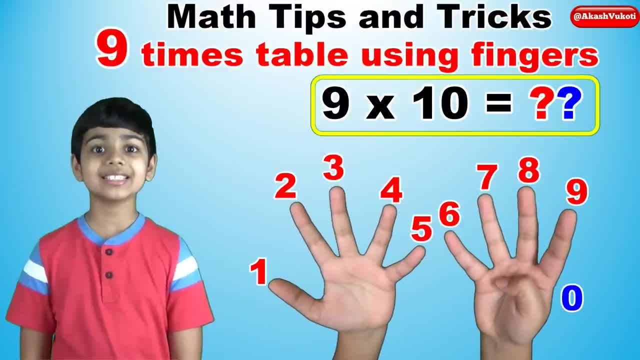 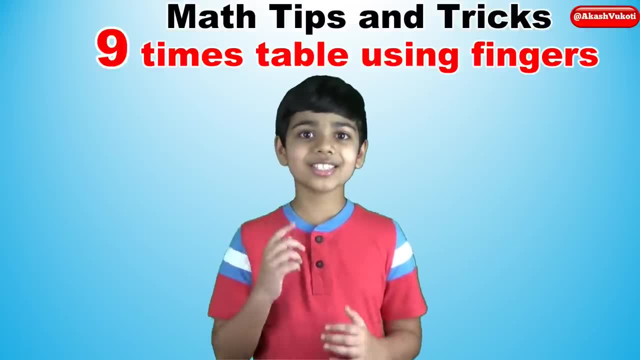 9, 2, 3, 2, 2, 1, 0.. 0. The answer is 9, 0, 90.. How cool was that right? This is the best trick to remember the 9 times.